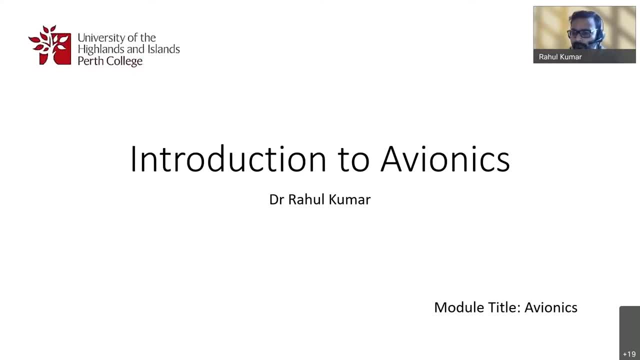 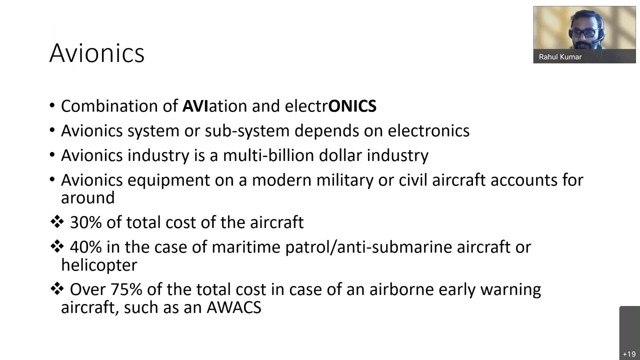 just to introduce you. And finally, we are going to study about the steps that are followed, or that need to be followed, for designing an avionics system. Right? So let us start with the avionics. What is basically avionics? 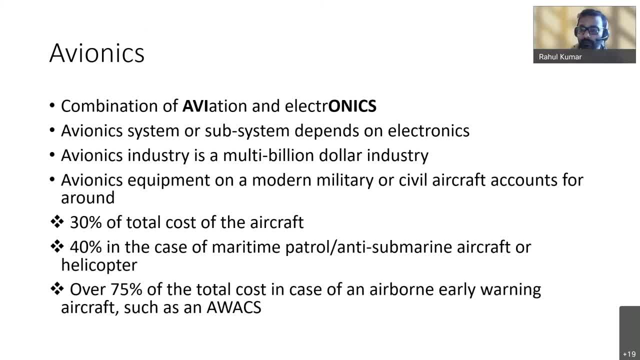 Right So the word avionics. it is a combination of two words: aviation and electronics. Right. So basically, in this module we are going to study about the electronics in an aircraft, Right So this word. it was first used in 1950s, long back Right, And since then the avionic. 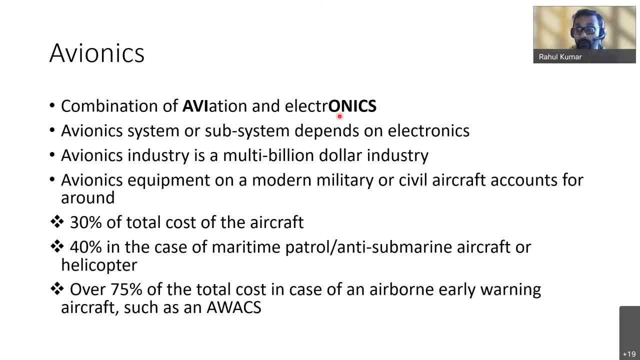 industry has developed quite a lot, Right, So we are going to study about the electronics in an aircraft, Right So we are going to use these- this word avionics, system or subsystem- quite a lot in our further discussion or in our classes. 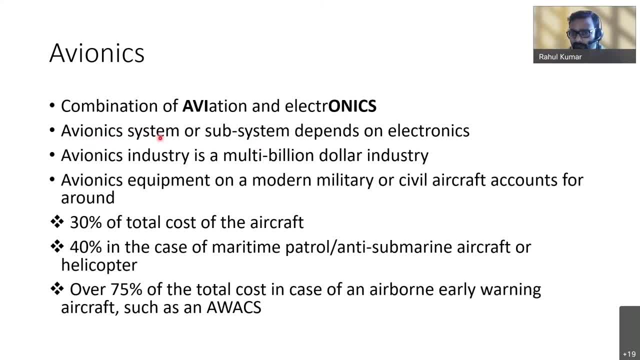 So, basically, avionic system or subsystem. this simply means that any system in the aircraft which is dependent on the electronics Right For its operational capabilities Right, Please hold on. So basically, it means thatmayae system or subsystem. this simply means that any system in the aircraft which is dependent on the electronics Right For its operational capabilities, Right For its operational capabilities Right. 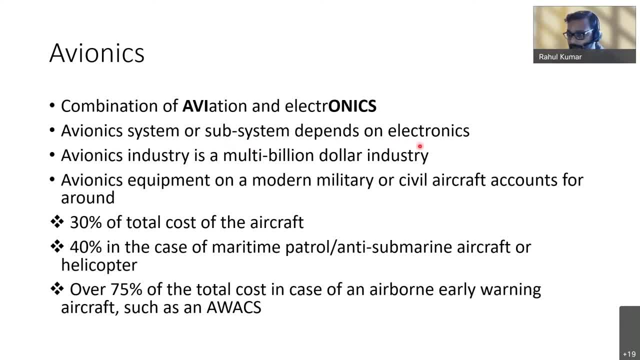 It means thatmayae systems, or electronic, are not primarily金 and black imaging, such as Schrödinger's and tãoah him remember. But in our lecture over is, or it can be categorized or called as avionic system, Although we are going to study some of the 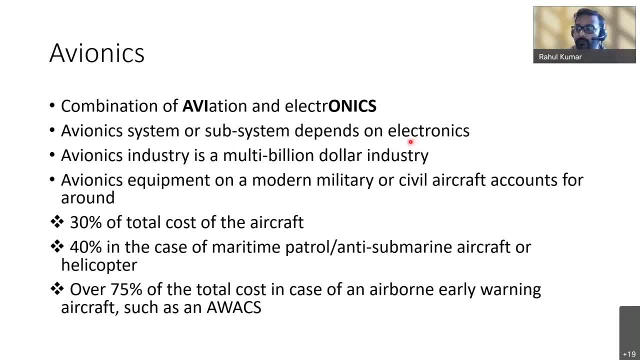 systems which will involve electromechanical parts as well. right, even then we are going to categorize them as avionics system or avionics subsystem. So in any system of the aircraft, if there is some part is electronic, we can call it as avionic system. Now, obviously we all must. 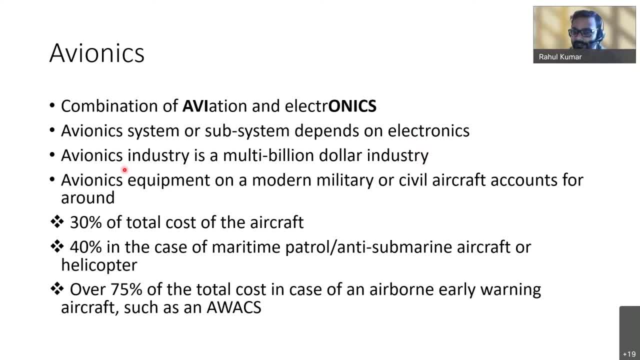 be aware that avionic industry is a multi-dollar industry and in most of the modern military or civil aircraft the cost of avionic systems which are installed on the aircraft it costs around 30% of the cost of the aircraft. So if there is some part is electronic, we can call it as avionic system. 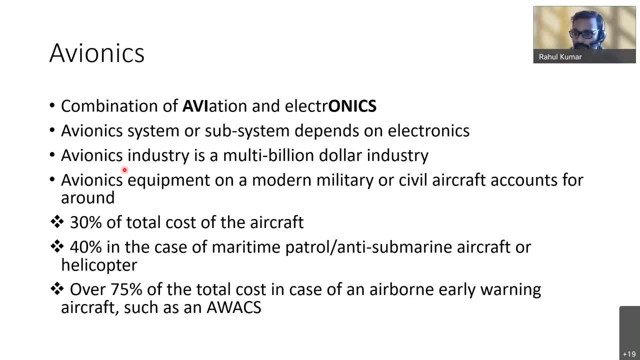 The cost of the aircraft is 40% of the overall cost of the aircraft. right, And in high-end or maybe some advanced version of the aircraft, something like maritime patrol or anti-submarine aircraft or even helicopters- right, they also highly rely or depend on these avionic systems. So for such aircraft, 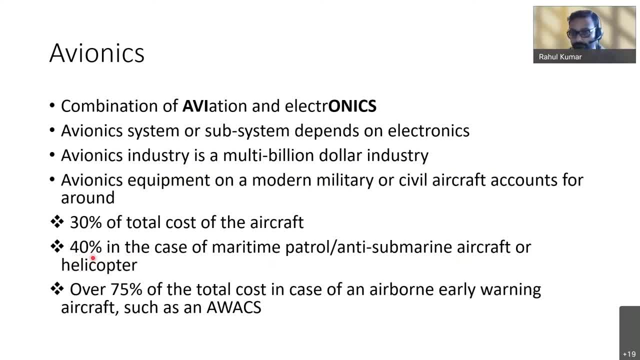 the cost. it increases to 40%, right? so out of the total cost of the aircraft, you are or the person is paying 40 percent just for the avionic systems which are installed in the aircraft. so you could imagine how big this industry is. and nowadays, in evac system or in unmanned air vehicles or aircrafts, the cost is 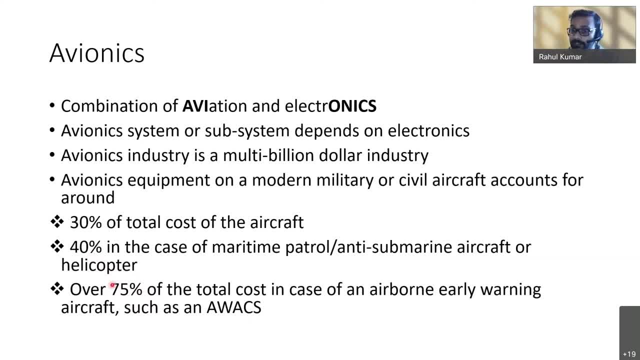 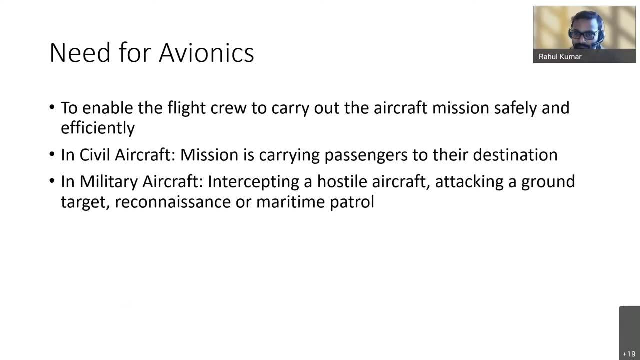 further, higher, it's more high. it's around 75 percent of the total cost, right, so you could imagine how big or how well developed or advancing this this industry is. now why do we need avionic systems? why do we need avionics in an aircraft? so, initially, 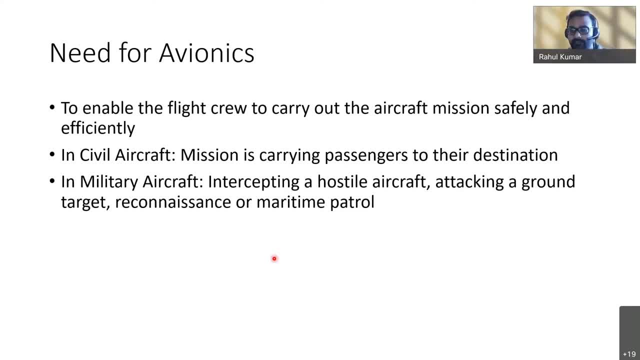 uh, these avionic systems. they were installed in the aircraft to carry out aircraft missions safely and efficiently with less number of flight crew, right? so that was the initial need for developing your avionic system. now you might. nowadays, basically in most of the civil aircraft, we only have like two flying crews or you have only two pilots. 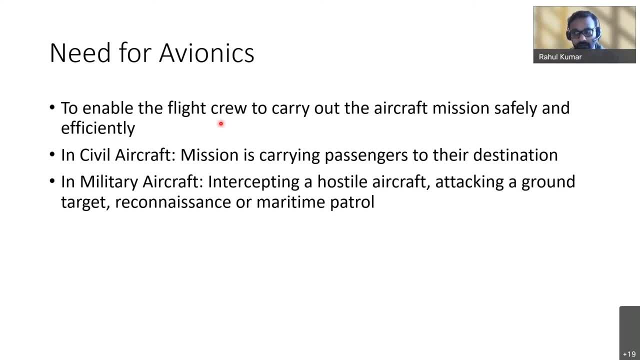 one is the first pilot and uh, or the captain and the second pilot, so you have only two people flying the aircraft. but in older days there used to be a crew member of four people, so you would have two pilots and a navigator and a aircraft engineer. so all together there were four people who were flying the aircraft. 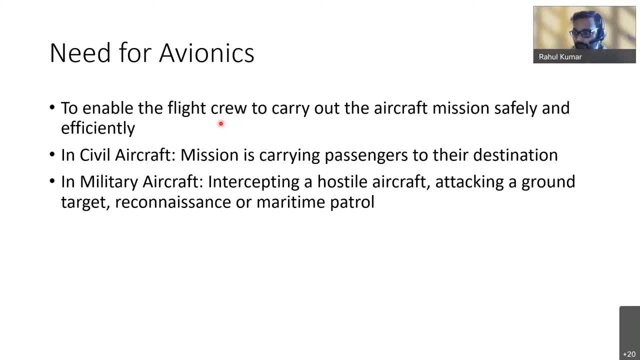 right. but with the development of avionic systems, uh, now the work of mostly the engineers and the navigator. it can be done by this: avionics installed in the aircraft, right. so now only two or two people are able to fly all the三 or four people who have the 선생님, the construction. 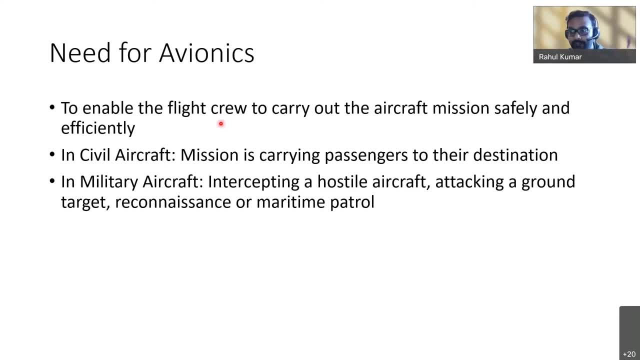 engineers, the DCV. they can also fly the aircraft, the yeah, but they were the cuánty right sample visible as well. then you also have a control system which, being vana err rightir, also a steering sensor, right, a steering sensor which is used for controlling the air force, HIS estudio. and then this is a pilot product that can be used in an other persongie: the pilots. they can fly the aircraft without the help of 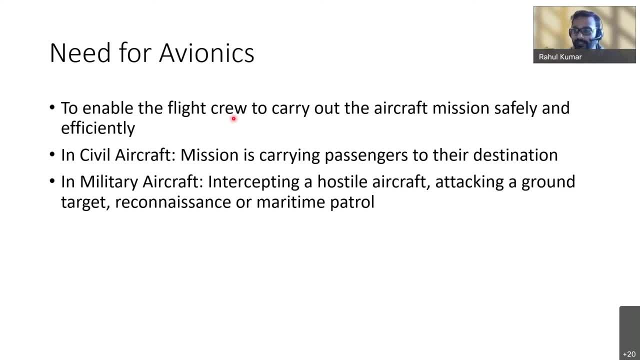 carry that weight. So if we can reduce the weight, we can carry maybe more number of people or passengers in the aircraft. So it has a cost benefit. If you reduce the weight, it has a cost benefit for you And in terms of military aircraft it would mean you can carry more amount. 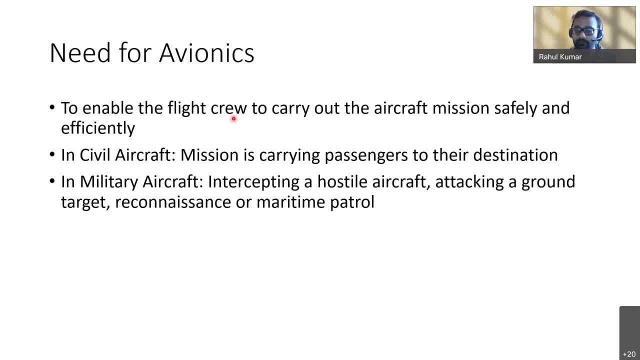 of load payload missiles or something. And also, if you reduce the weight, it would also mean that you can fly for longer duration, right? Because you have to burn less fuel to carry that lighter weight. So obviously all these were the advantages which helped in developing this. 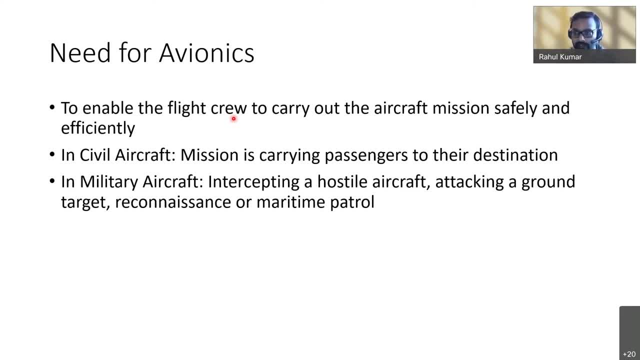 avionic industry And we all can see that almost nowadays, 70%, or at least 40 to 50%, of the cost of the aircraft is your avionics system. Now the avionics system are used to carry out aircraft missions safely. 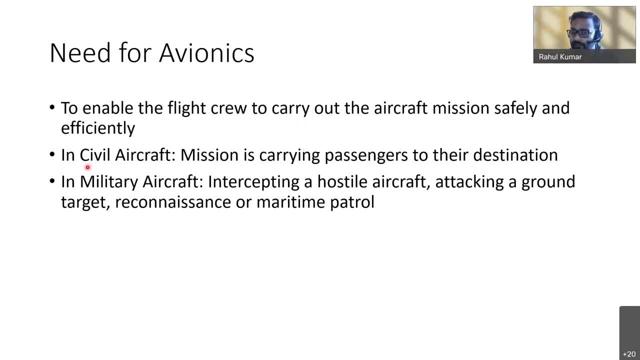 So what do we mean by mission? So, in terms of civil aircraft, your mission is to carry passengers to their destination. In terms of military aircraft, it would mean either intercepting a hostile or enemy aircraft or attacking the ground target, or maybe just patrolling or surveillance of the area. So that is what it means by mission: aircraft mission. 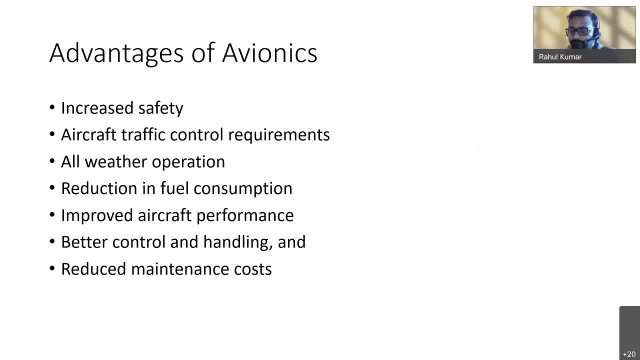 Now coming on to the advantages of avionics systems. So obviously some of the advantages we have discussed just now, right. So along with those advantages- the avionics system- they have several other advantages With the use of avionics system. obviously there is increased safety, or the safety of the aircraft is. 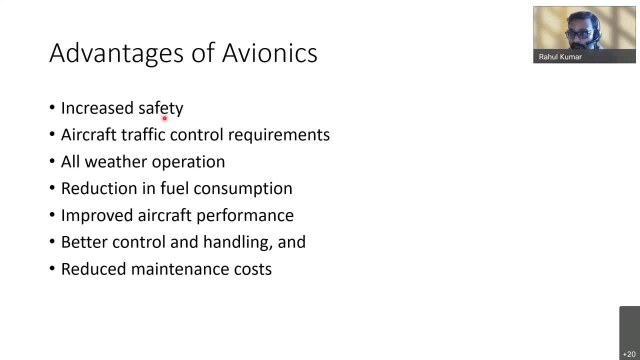 increased. now There are less number of accidents. The second advantage is aircraft traffic control requirements. So for ATC: now you can track the aircraft and you can manage all the aircraft Right, Right. So for air traffic controller: they can track and monitor the aircraft. 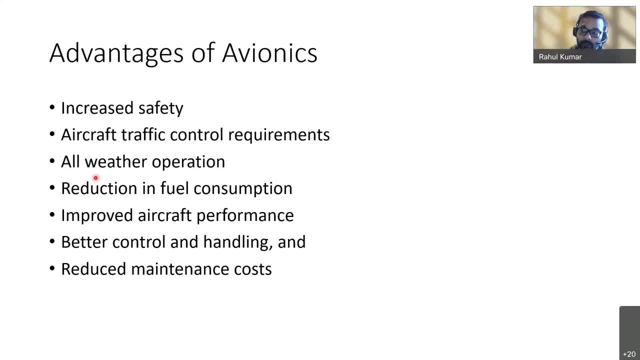 All-weather operation again. in older days the aircraft could only fly in a better visibility condition or in daytime, But now with the use of avionics system, like certain radar and night vision, so it provides better visibility to the aircraft, Like radar and night vision also, you can operate good� play at youPM 17 shark. 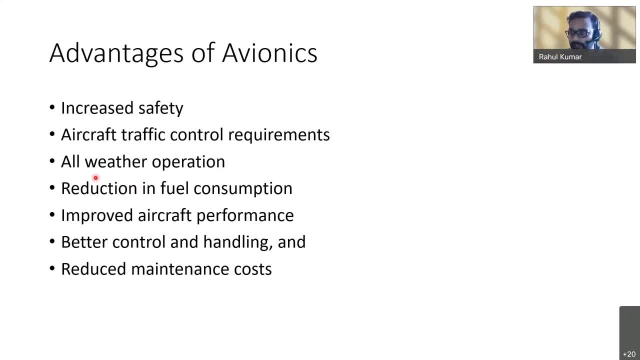 the aircraft in all weather condition and even in the night time, also in dark. also. reduction in fuel consumption. again, there are systems to monitor the engine performance and they also monitor the fuel consumption. so it optimized or it improves or reduces the fuel consumption as well. improved aircraft performance. so 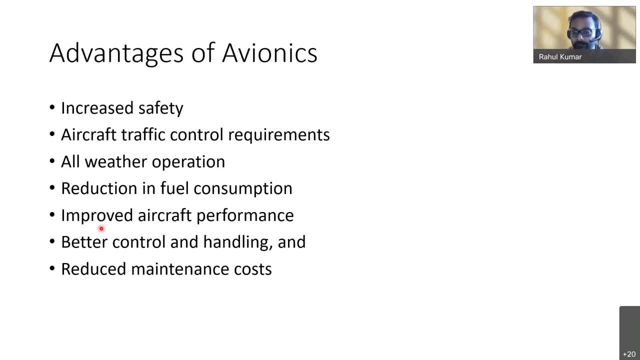 obviously, all these factor would definitely improve the performance of your aircraft. and the other advantage is better control and handling. so you have so many avionics system which something like cruise control and automatic landing system, right? so all those avionic system. they enable the pilot to 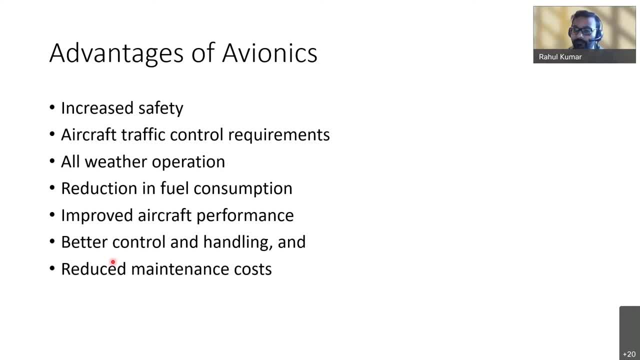 control the aircraft in a better way it is. it is making the control of the aircraft much easier for the pilot and reduced maintenance maintenance cost. so again, you have some avionic systems which monitor all the parts of the aircraft and if it needs any kind of maintenance it will give the specific 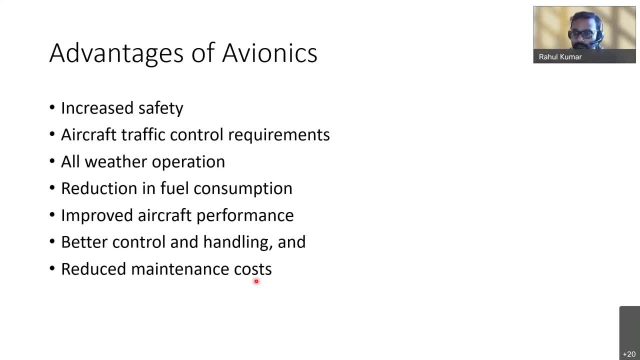 requirement or the maintenance requirement to the maintenance engineer. so you don't have to, or the maintenance engineer does not have to, look for the problem, it will be the avionic system gives the problem to him that you need to replace this particular part. right, so the maintenance cost of the aircraft is. 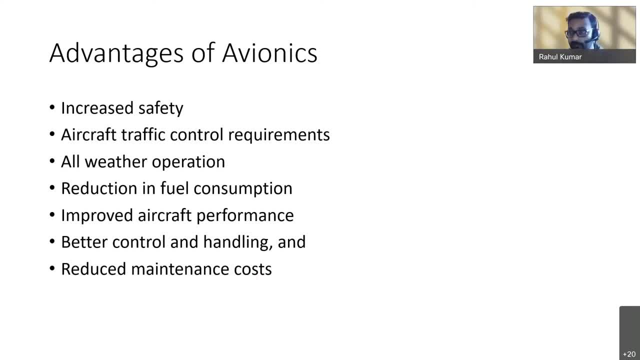 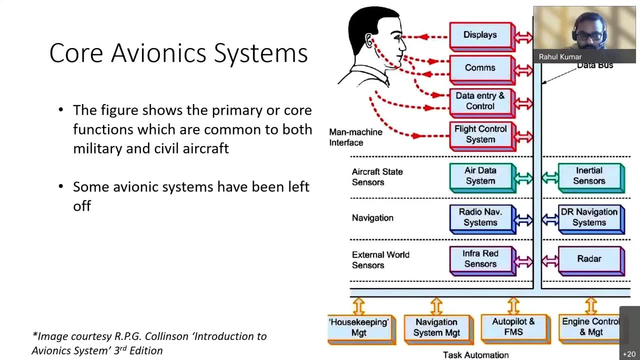 reduced and the cost is also reduced and the time is also reduced. now coming on to the next slide. so this picture in the slide, it kind of represents the core avionic systems, right? so the figure shows the primary or the core functional functions which are common to both military and civil aircraft. however, 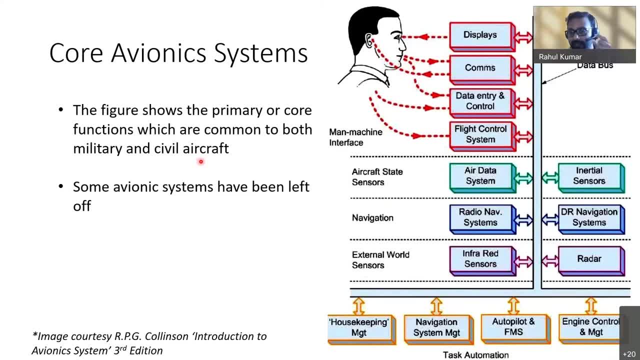 there are some parts or some avionic systems which are missing in this diagram. right, for example, you have ground proximity warning system. it is the system which sounds pull up, pull up when the aircraft is near the ground. so it gives audible or voice warning, right? so, or maybe your? 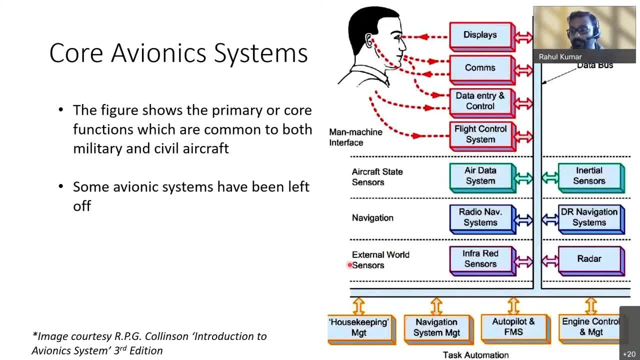 air traffic controller or ATC transponder system is another important part which is used in most of the aircrafts right, which is not represented here. so although this picture it represents of the core avionics system, but some of the avionics systems they are missing. 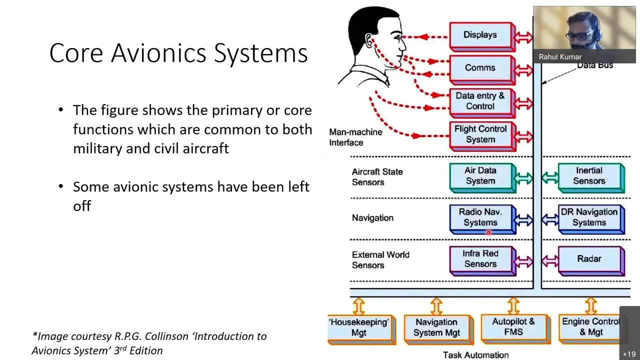 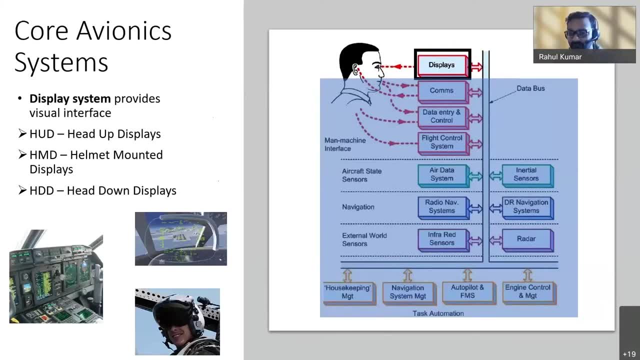 they are not represented in this picture, But obviously this was the best one which I could find to give you an overview of the different avionics systems, so I'm using it. So, to start with the different core avionics systems, the first one, or the first few, are the ones which the pilot can see, or you can. 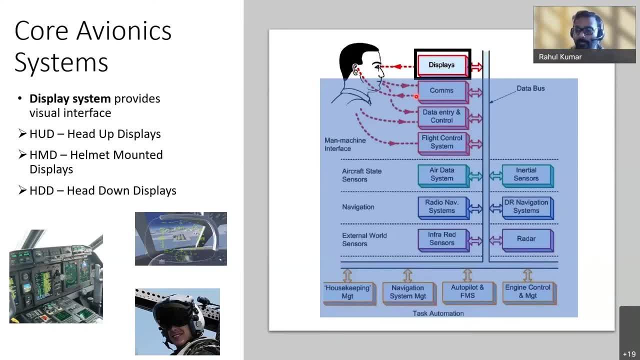 visually see them in the cockpit. So the first one is your display system. So obviously, when you walk into a cockpit you would see some display, lots of display, basically right. So displays: they provide visual interface and they can be of three types. so you 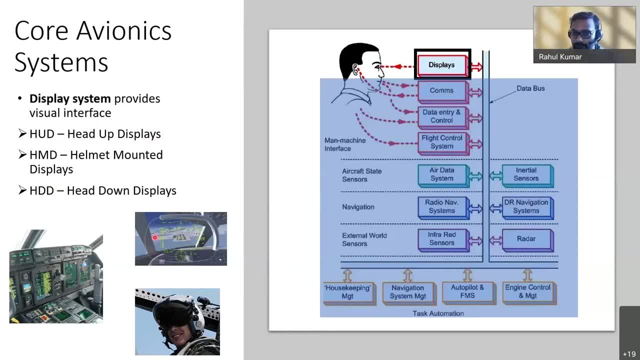 have head-up display, so this picture is for head-up display. so, as you can see, like while looking for information, the pilot is not able to see it at that time. pilot doesn't need to look down. The pilot can keep his head up and he or she will get. 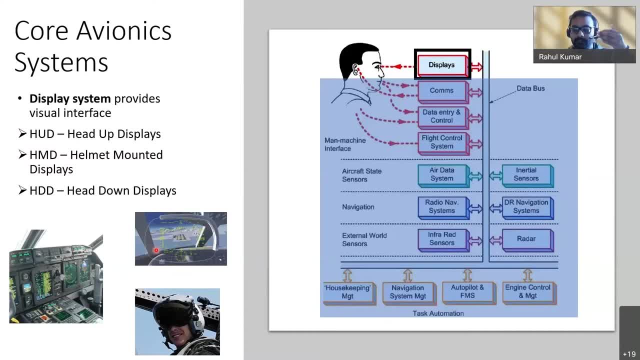 access to all the information. So, basically, this head up display is a glass on which the information is projected, and the glass it is transparent, so you can view the outside environment through this glass. So, along with the information, you would have situational awareness as well. You can look around the aircraft. you don't need to look down. 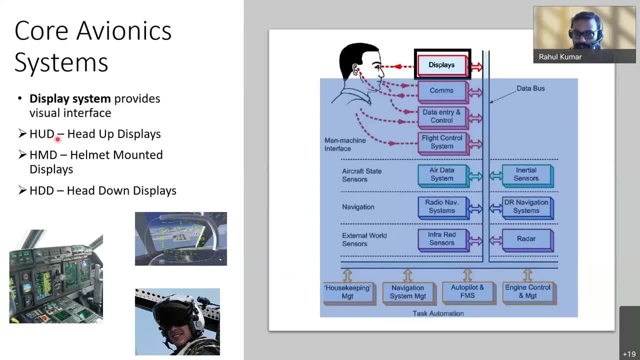 Right, so that's your head up display, or in short, HUD. The second type of display is called as helmet mounted display. So this picture is for helmet mounted display. So in this display the information is projected or displayed in the visor of the helmet. 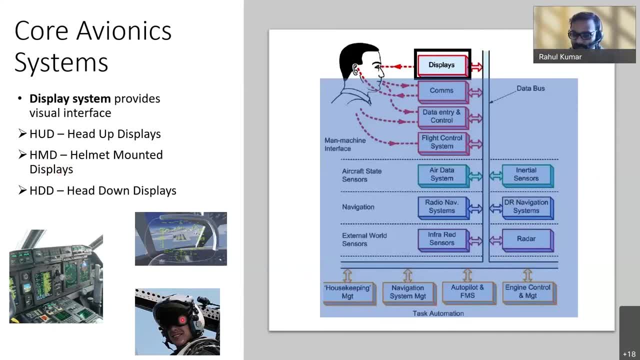 Okay, in this visor of the helmet, and so mostly it is used in helicopter, where the pilot wears a helmet, or maybe in military aircraft. They are not quite common in civil aircraft. In civil aircraft you use head up display, Okay, and then you have head down display, So these are your head down display. 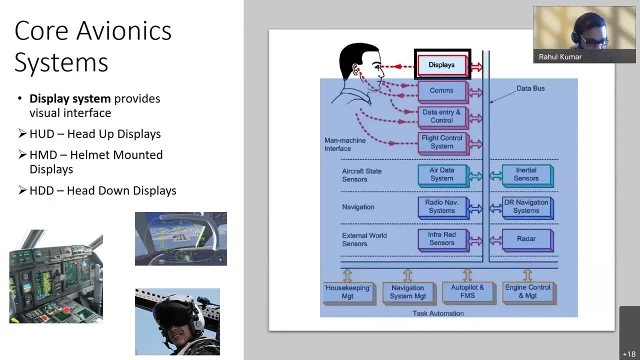 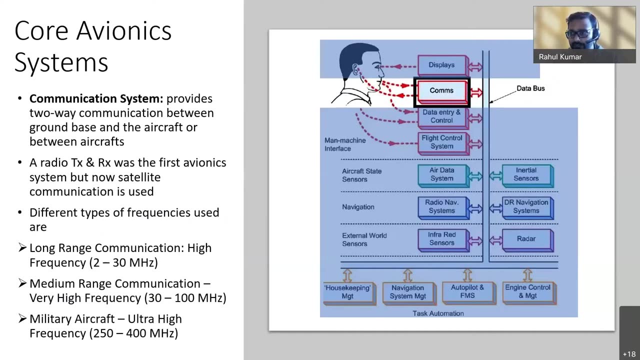 So if you want to access any information, you have to look down into the displays. Okay, Okay, so we are going to study about that. Okay, so we are going to study about that. Okay, them in detail in the future classes. The next type of avionics system is your. 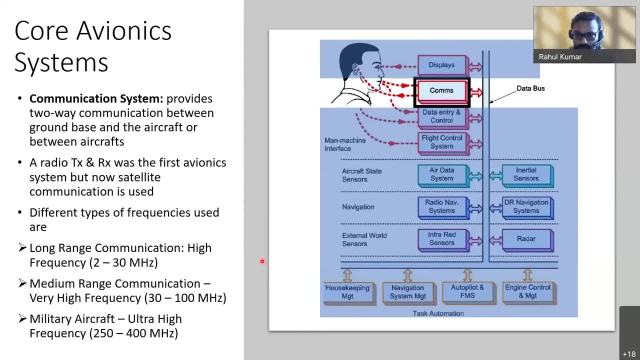 communication system. So again, you would find some radio set in the in the cockpit over which the pilot can communicate, so that can be also easily seen by the pilot or it is visible. So the communication system provide two-way communication between ground base and the aircraft or between aircraft in the. 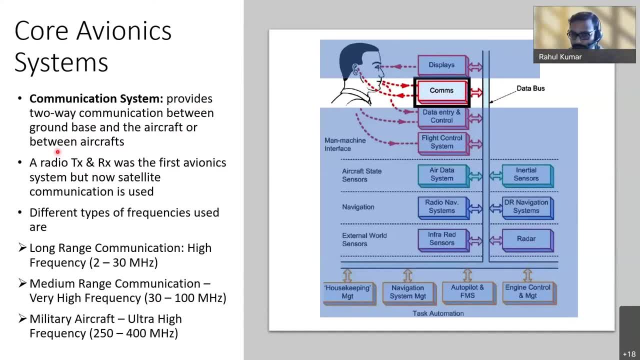 surrounding between two aircrafts also. So the first avionics system was simply a radio transmitter and receiver, But nowadays we have several satellite communication as well. right, So most of the aircraft they are now fitted with GPS system and satellite communication systems as well, But in older days we only used to have this radio. 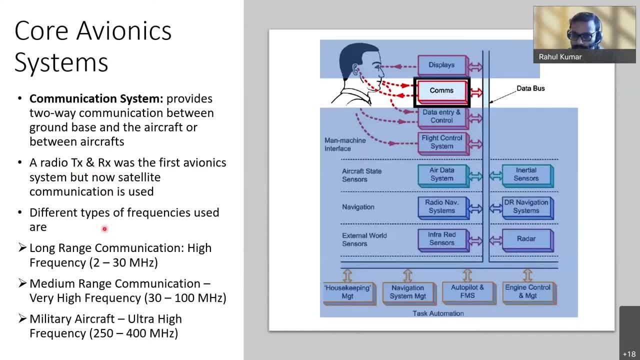 communication, only The communication systems. they use the radio communication, only The communication systems. they use The communication systems. they use different frequencies. So for long range communication we use high frequency, somewhere around 2 to 30 megahertz. For medium range communication we use very 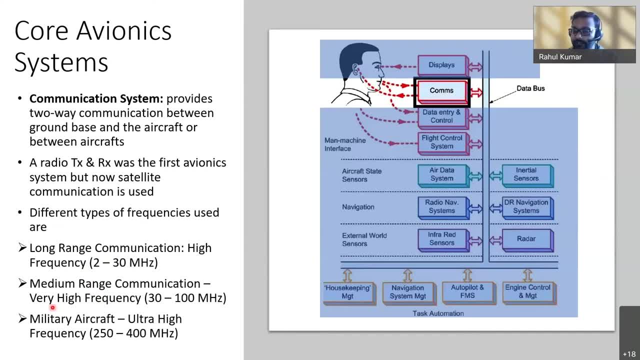 high frequency, or in short, we call it as VHF, very high frequency communication, somewhere around 30 to 100 megahertz, For medium range communication. we use very high frequency, or in short, we call it as medium range communication, Maybe communicating with other aircrafts, And 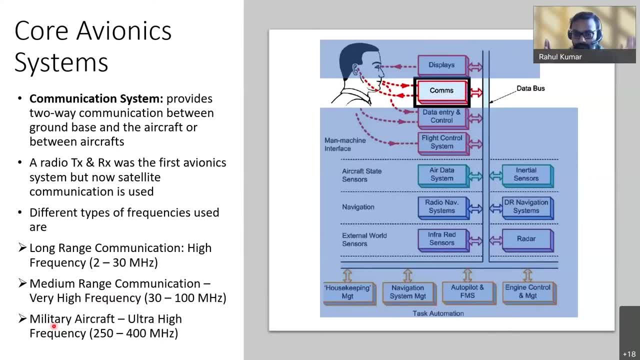 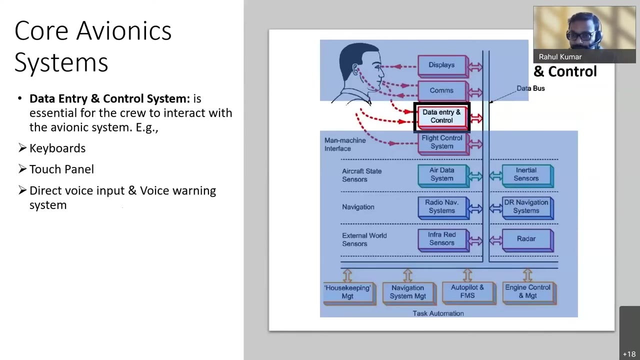 for military aircraft you have a dedicated frequency band so they use ultra high frequency, around 250 to 400 megahertz. So again, we are going to study about the different communication system in detail in our future class. The next type of avionics system is your data entry and control system. So 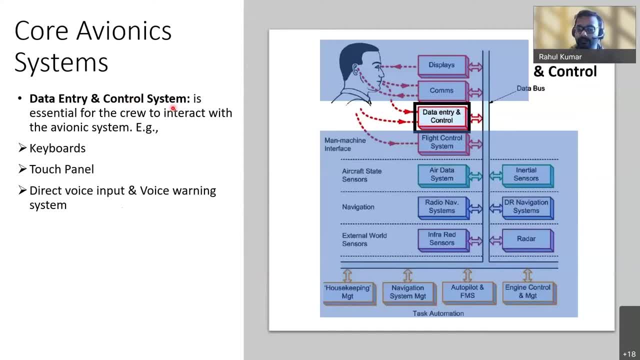 obviously to feed in the data you would need some keypad, some touch panel right to get the information. So data entry and control system is essential for the crew to interact with the avionics system. So some of the examples are keyboard, touchpad and direct voice input are also being used. Maybe you can at the 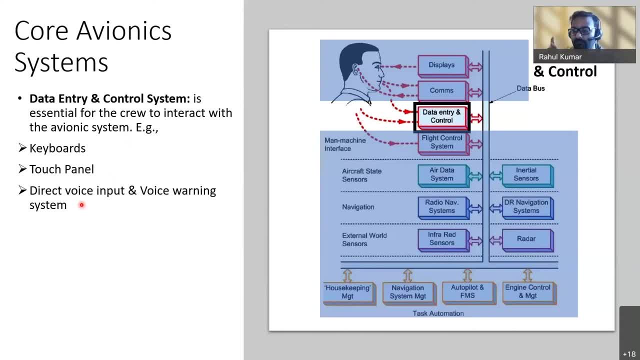 pilot. they can use some phrases or some words as a as an input. But obviously everyone they have a different, maybe accent voice, speech, speech, speech voice. So they are not very common direct voice input. But yes, such type of system is also available. right, And voice warning system are also there. So with 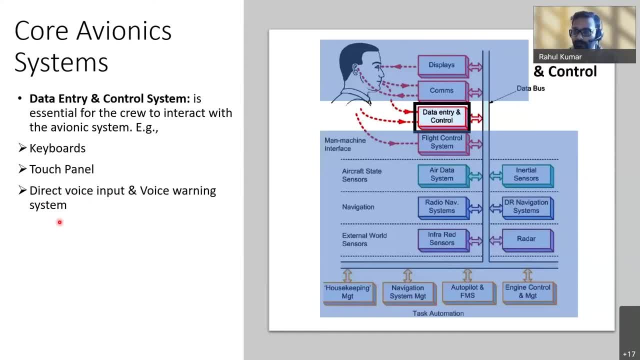 along with with the visual display, you would also hear some voice or some warning right? So something like the example I was giving: pull up. pull up So that sound or voice warning system is also being used in the avionics system. So 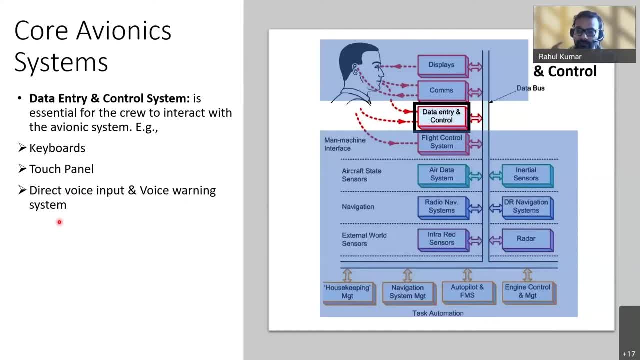 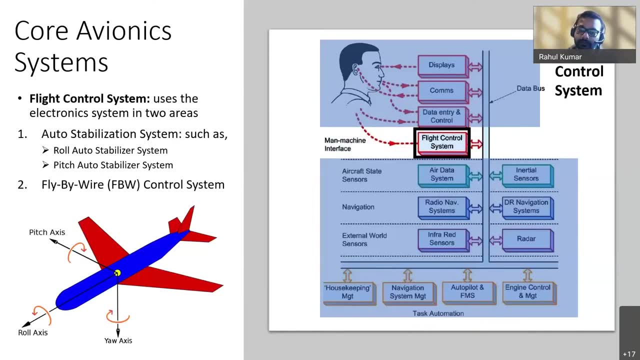 that is given by voice warning system. that is given by voice warning system, right. The next avionics system is your core avionics system. sorry, is your flight control system right? And they use the electronic system in two areas, right So? 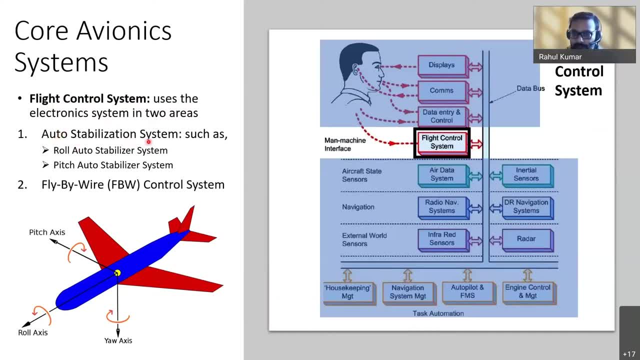 one is you have to use your auto- stabilization system and fly-by-wire control system. So auto stabilization system, such as your roll auto stabilization system, which damps or suppress the motion about the yaw axis and the roll axis of the aircraft. Similarly you have pitch auto stabilizer system which suppresses the short periodic motion. 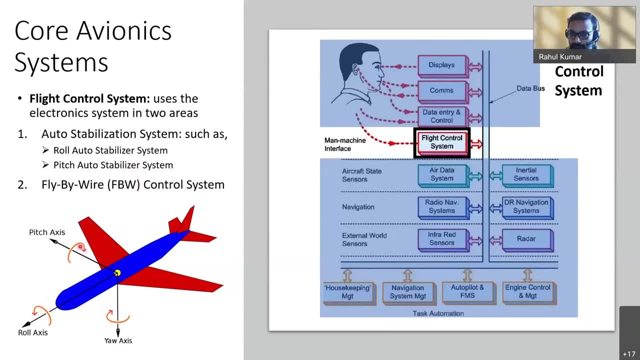 between the pitch axis. So basically these two subsystems are used to stabilize the aircraft in flight or in air so that it doesn't topple or it doesn't move, to provide a better control of the aircraft. So generally in most of the aircraft you would need both or control over all the three axis. 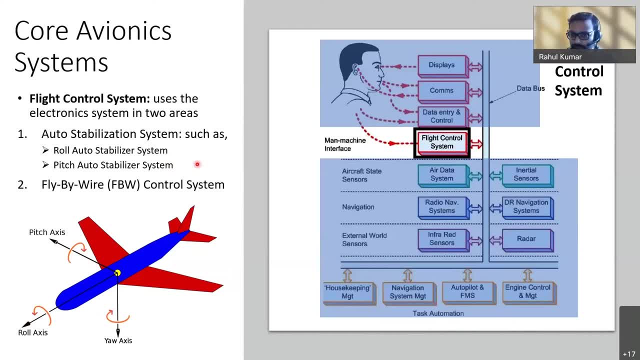 for better stabilization. Then you have fly by wire control system Which provides continuous automatic stabilization of the aircraft, And they use some motion sensor to stabilize right. so with the help of several sensors which are installed in the aircraft, you maintain or automatically the aircraft is stabilized. 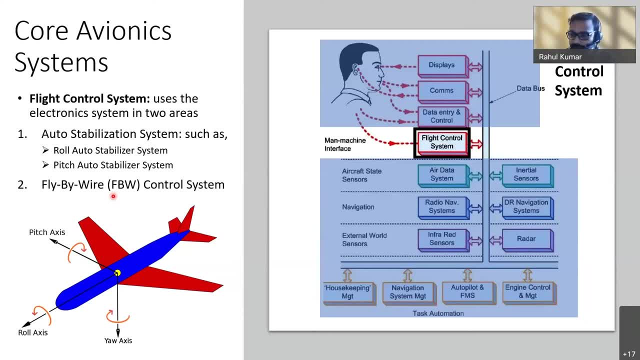 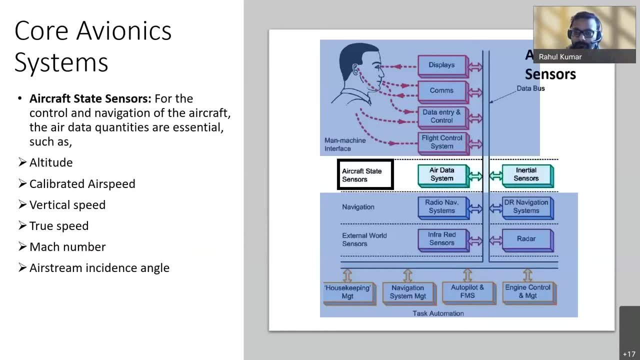 or its stability is maintained. The next type of avionics system: they are called as aircraft state sensor, right so these are used for the control and navigation of the aircraft. So So, Like in the previous slide, I was just mentioning that, with the help of some sensors, right you? 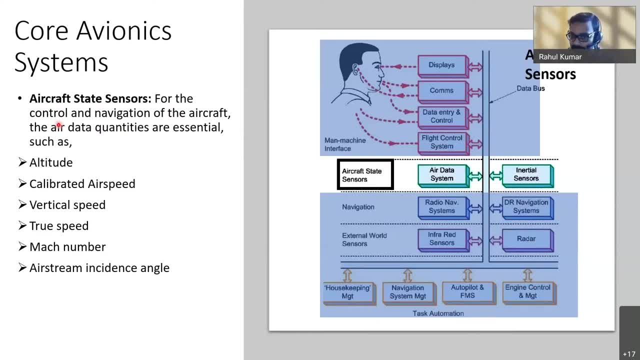 would maintain or stabilize the aircraft in the air. along with those sensor, you would also need some air data maybe. what is the wind speed, right? what is the pressure being exerted on the aircraft, right? So all those information, they are collected by air data system or again you have a separate. 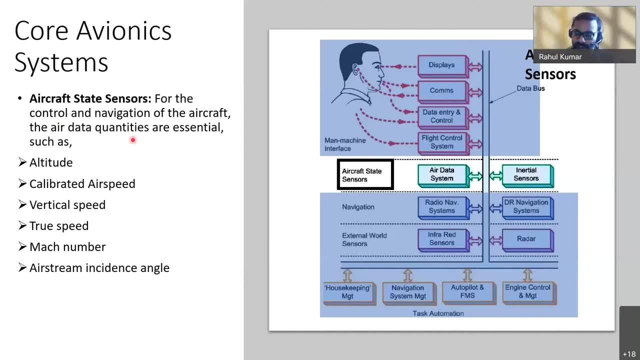 set of sensors which collect those information and these air data. they can be used to calculate the altitude, the air speed, the vertical speed and usually in the military aircraft which fly at a speed, So The altitude which flies at a speed around the speed of sound. so you can even calculate. 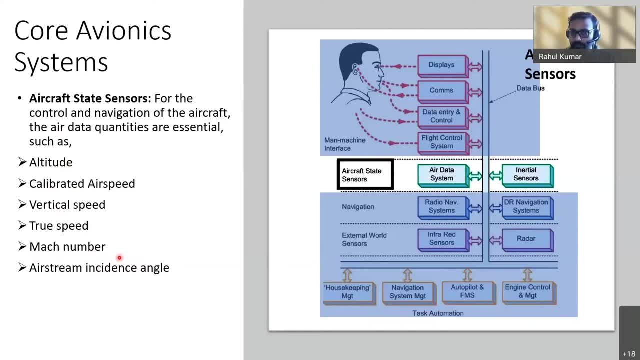 the Mach number or Mach speed of the aircraft. So, again, with the help of aircraft state sensor, you can calculate these values. ok, Hopefully in the last unit. The last unit is on air data indicators, right, So in that unit we are going to study about all these different indicators, altimeter and all right. So we will study the working principle, how, with the help of pressure sensors, temperature sensor, how we can calculate the altitude, the airspeed and the Mach number of the aircraft. 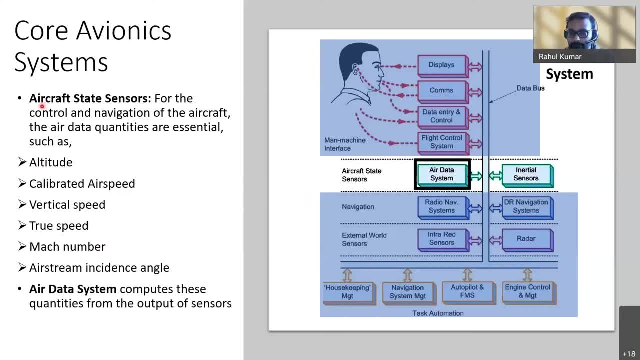 So in this aircraft state sensor, you have several subsystems, So one of the subsystem is your air data system, So, which is essentially a computer connected to different sensors, right? So it collects the information from the sensors, process it and provide the air data information. 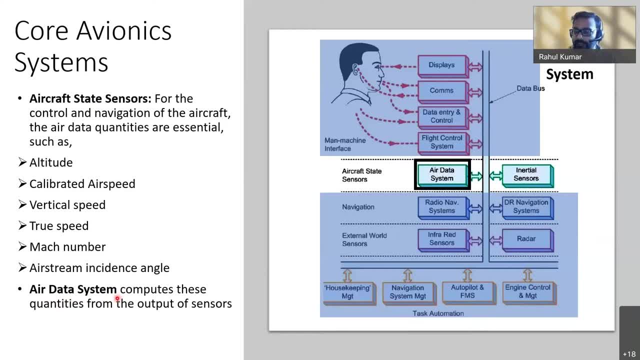 Again, as I mentioned, it will give you the temperature, the atmospheric pressure and all those information about the air, or it will give you that information about your surrounding of the aircraft And obviously they can be used to calculate the altitude, the speed and the Mach number. 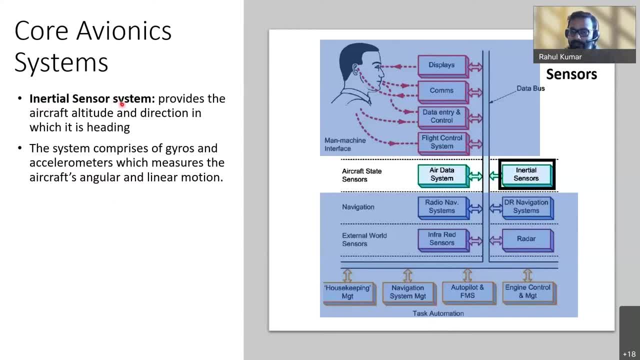 Okay, Okay. The next subsystem is your inertial sensor system. So these inertial sensor system, they provide the aircraft altitude and direction in which it is headed right, And basically, these sensor, they are your gyroscope and accelerometer. Those are called as your initial. 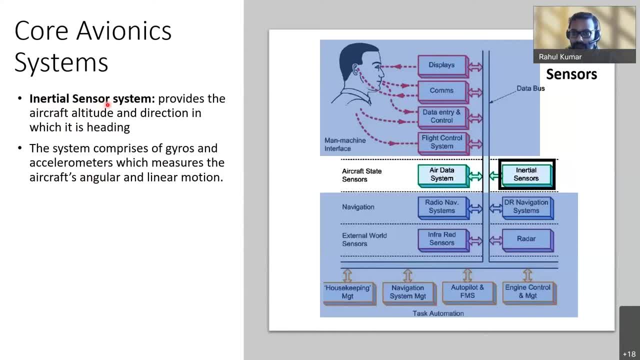 So these are called as your initial sensors. Okay, So, with the help of these inertial sensors, your gyroscope and accelerometer, you can identify the location of the aircraft. Okay, So, in the future classes we are going to study about inertial navigation system. 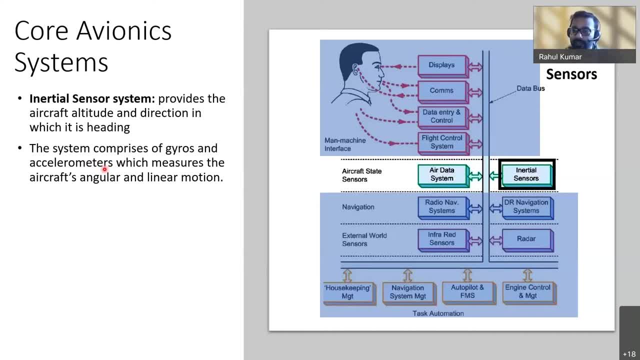 Okay, So the benefit of this navigation system is that it is independent. Okay, Okay, right, it can work on its own, it doesn't need any like gps system or like that right, it can individually give the location or the position of the aircraft with the help of the inertial sensor. 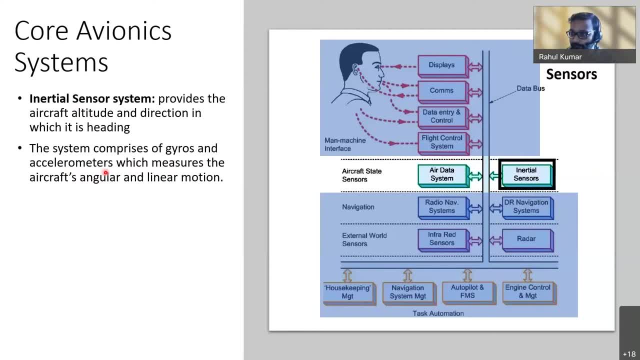 your gyroscope and accelerometer right to gyroscope it will- uh, it gives information about the angle at which the aircraft is flying, and accelerometer it will give the speed of the aircraft. so if you know at, if you know your reference point, so like if you are, if your. 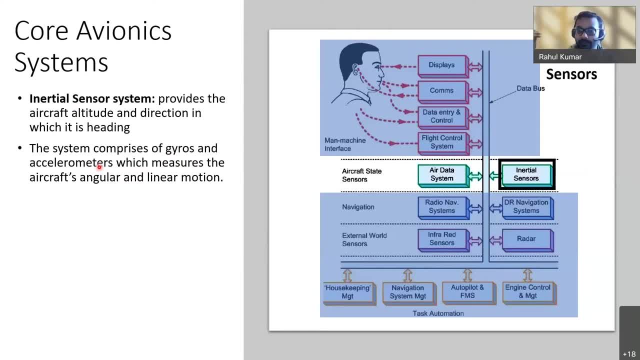 aircraft is flying from beijing right and it is flying at this angle and at this speed right, at 30 degree angle and maybe 100 knots right. so you can identify that after one hour of flight this is the speed of the aircraft flying from beijing. so if you know if your aircraft is flying from beijing, 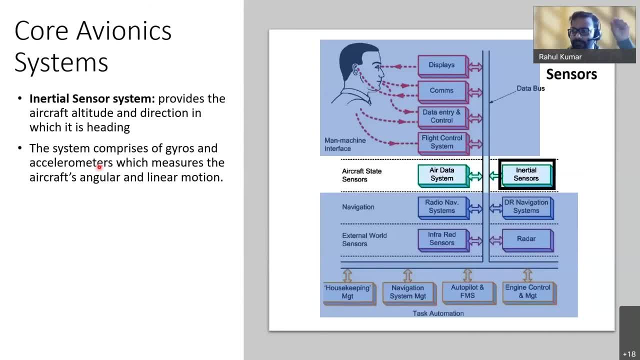 will be the location roundabout or approximately. this will be the location of my flight, right? so since it does not depend on any other system, it works independently. so it is quite useful just in case if your GPS system or your satellite navigation it is not working right, so you can use the inertial. 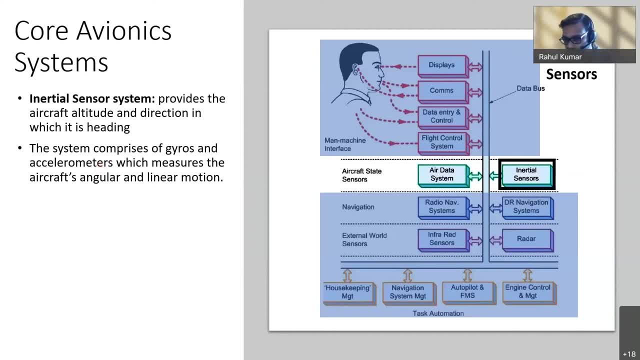 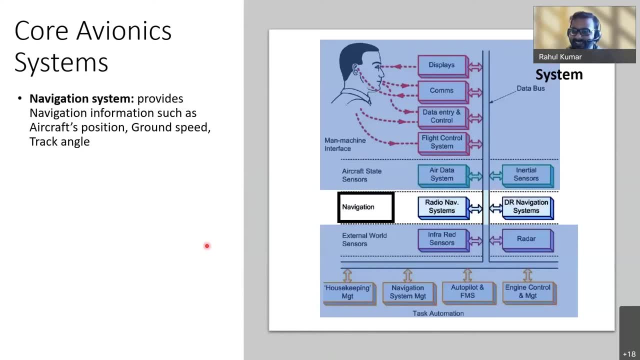 navigation system. okay, so coming on to the next avionics system, which is, which is your navigation system. so, navigation system, it provides information, navigation information such as your aircraft's position, ground speed and tracking, so it gives all these three informations. the first type of navigation system is: 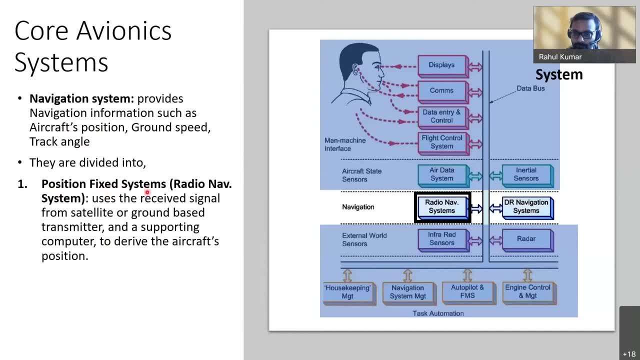 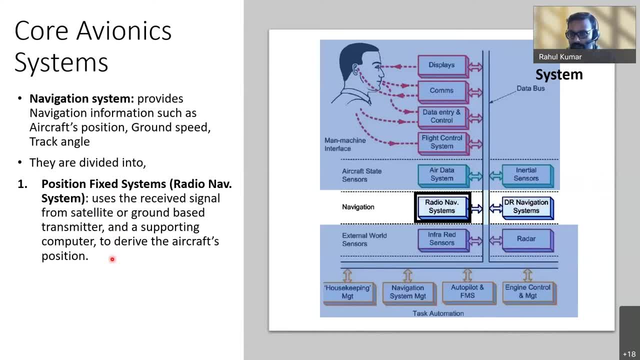 near your location. so there are two options: either you will ask someone that where is that particular restaurant, or you would simply, if you have an idea, you or you would simply, if you have an idea. you would continue moving in that direction and maybe estimate that after like five minutes. 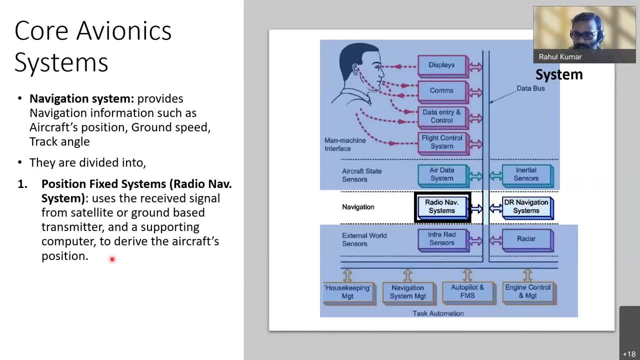 I should reach the restaurant or that place. So, if you are asking someone, that is similar to your radio navigation. So you have GPS systems, or you have ATC's air traffic control systems, and also you have VOR systems as well, So which provides the exact location of the aircraft through radio communication. 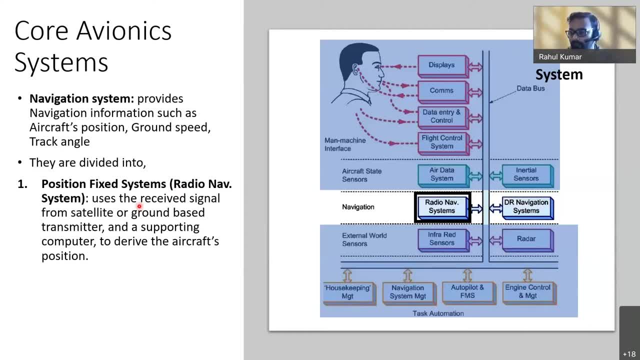 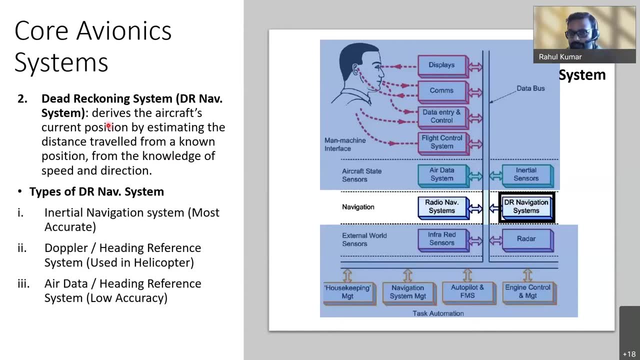 It will tell you that this is the exact location of your aircraft. The next type of avionics system is your dead recording system, or in short, we call it as DR Navigation. So this is the second type of navigation where you will continue to move in a particular 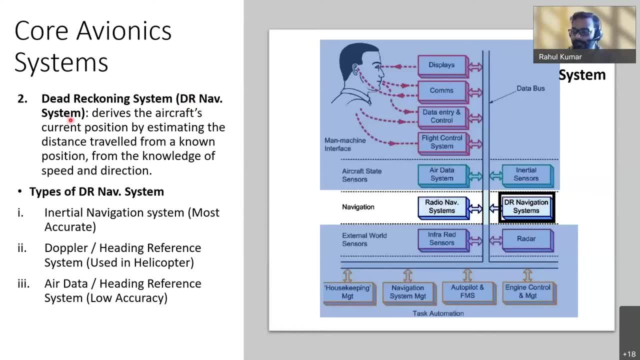 direction and you can estimate your location. So one of the navigation system which we have just now discussed is your inertial navigation system. So with the help of some sensors, basically a gyroscope and accelerometer, You can estimate or you can find the location of your aircraft. 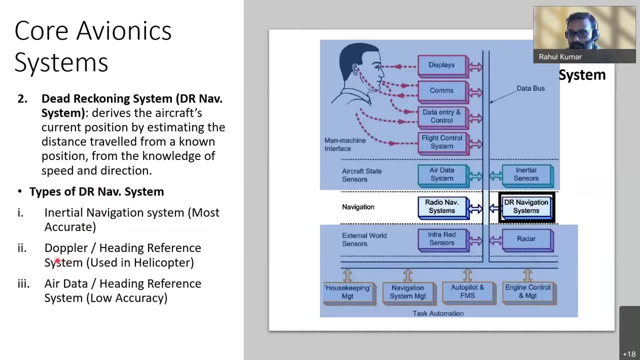 The second type of DR navigation is your Doppler or heading reference system, which are usually used in helicopters, And then you have air data and heading reference. So heading reference is, obviously, if you know your heading reference And you know the speed of the aircraft, so the air data will give you the speed of the aircraft. 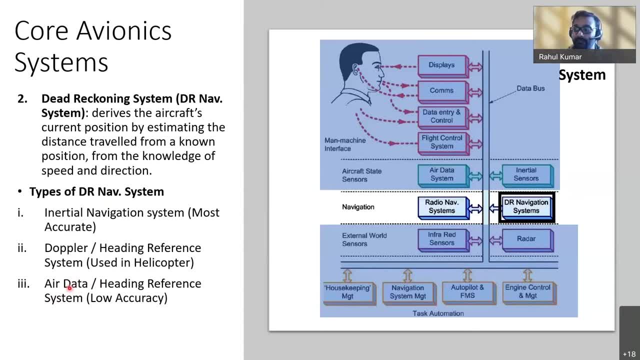 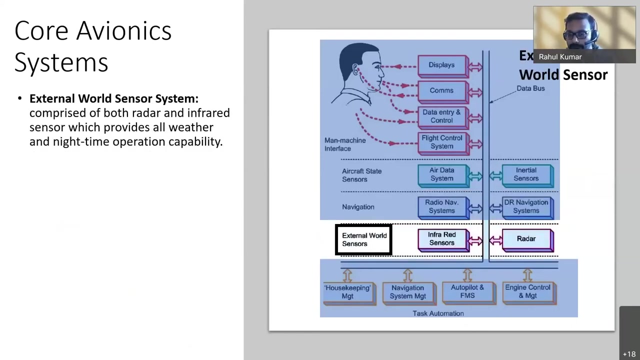 and all those information. so again you can estimate the location or the position of your aircraft. but the third option, or your air data and heading reference, it has very low accuracy. okay, the best one is your inertial navigation system. it has the highest amount of accuracy. the next type of avionic system: they are your external world sensor system. 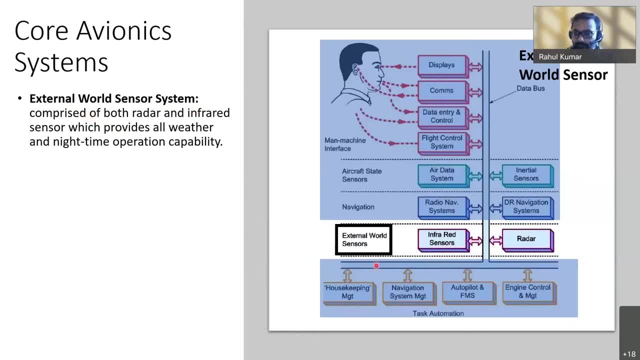 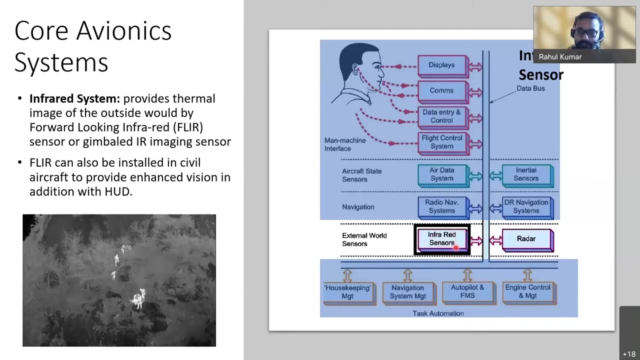 right, and they basically comprises of your infrared sensors and your radar which allow the aircraft to fly in different weather conditions and even in night time- okay, even in dark also, the flights or the aircraft can fly. so the infrared sensors and these sensors. obviously, i think you all must be aware about the infrared sensors, what they are. 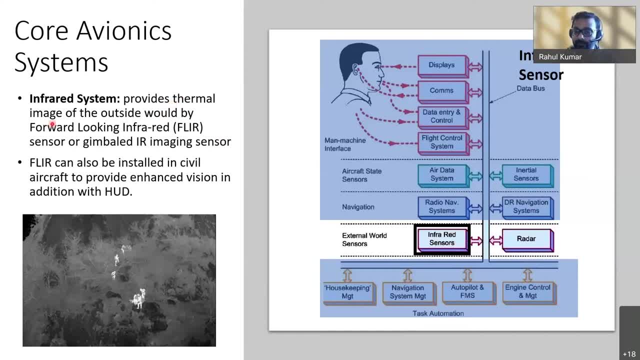 used for. so, basically, they provide thermal image of the outside world, something similar to this one. so, basically, your infrared system. they capture the, the heat source, and they like represented by a different shade of gray, something like the mid light silver, So the pilot can identify the object even in dark or in night time. 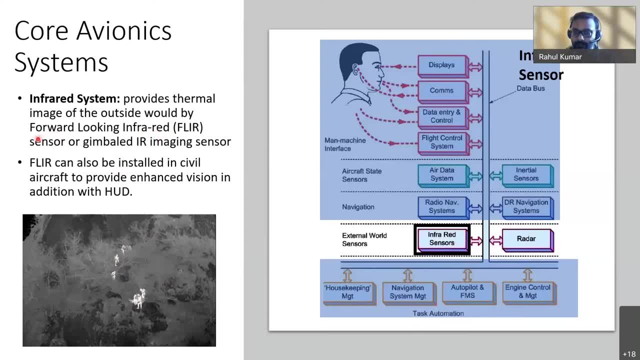 also So generally we use forward-looking infrared sensors for this, or sometimes we use gimbal in infrared image sensor to get this type of image in the dark- and they are generally used in military aircrafts, mostly in helicopters and some and even in like fighter aircrafts as well, to get a clear. 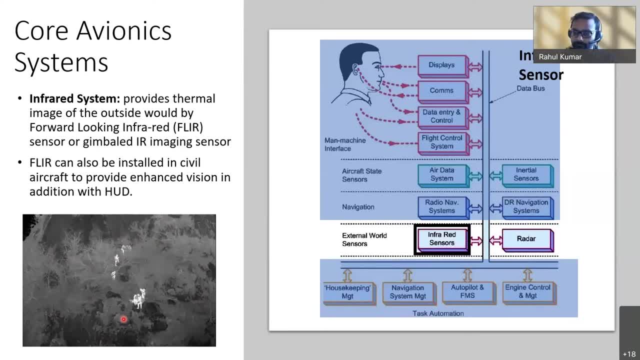 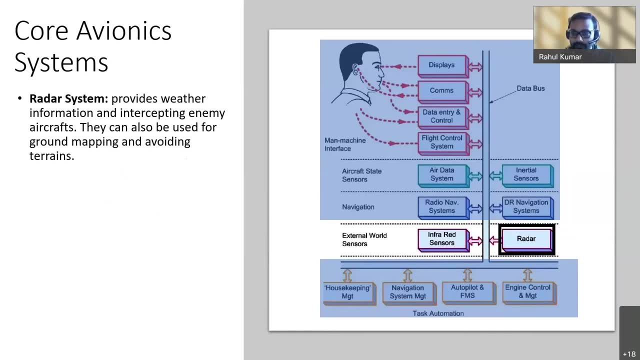 picture in the dark. And the next subsystem is your radar system. So obviously we all know what is a radar. in brief, We all know that they could be used to determine the weather condition. So radar system, they provide weather data or weather information, like whether it is cloudy or 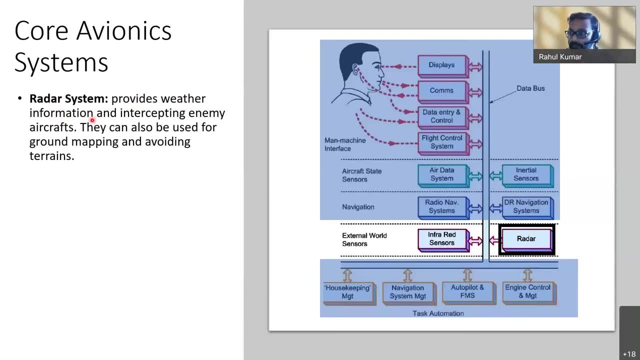 what is the condition in front of the aircraft if it is going to go through some clouds or maybe some bad weather condition. So the radar system will provide the information or the warning to the pilot. So generally we use multi-mode radar in the aircraft and along with the weather information or 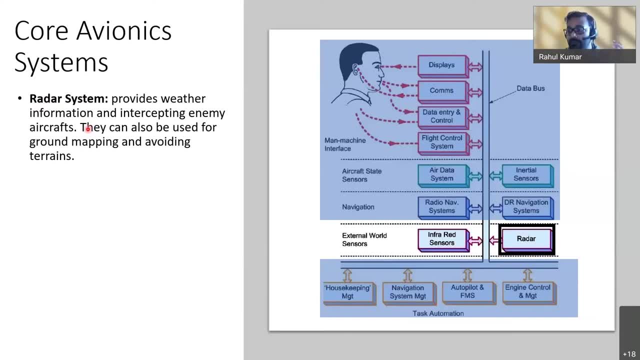 weather condition. these multi-mode radar they can be used to, you know, detect targets up to like 12 number of targets. and in the case of military aircraft, you would also need to track different aircraft, or maybe some hostile or enemy aircraft which are coming in. so with the help of radar system, this multimode radar, they can track up to 12. 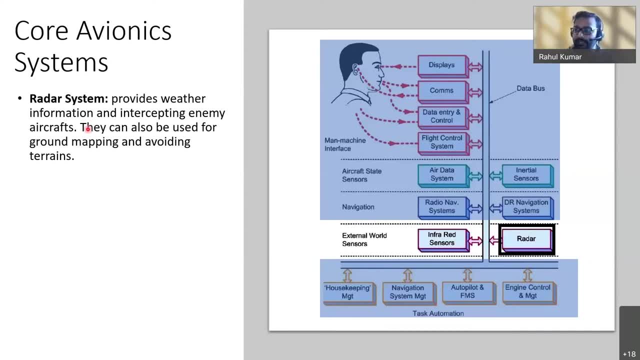 aircraft simultaneously and they can track the target or those hostile aircraft up to 100 miles away from the aircraft. so we use this radar system for two purpose: one is your weather condition and the second is for tracking right, tracking different aircraft. now the last avionics system is called, as your task, automatic systems and they are basically: 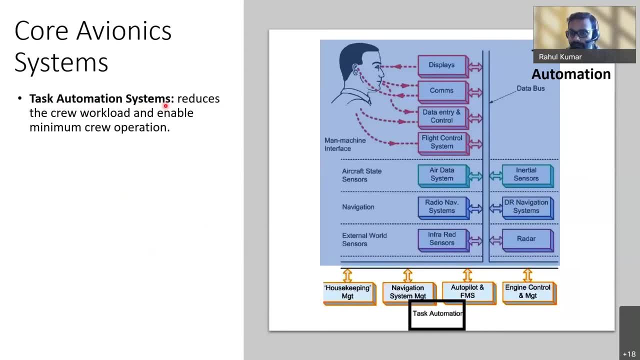 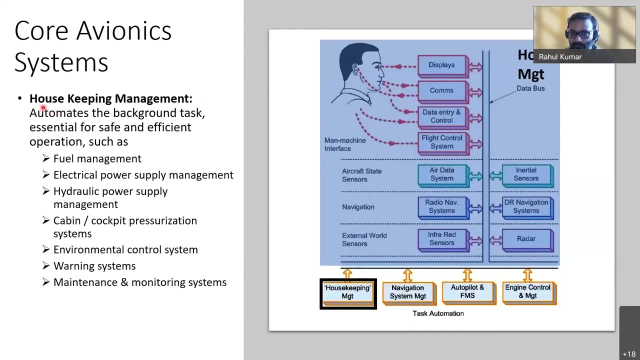 used to reduce the workload of the crew. okay, so you can operate the aircraft with minimum crew. okay, there are some subsystems. so the first subsystem is your housekeeping management. right, they basically automate the background task which are essential for safe and efficient operation of the aircraft. so, for example, you have fuel management system. 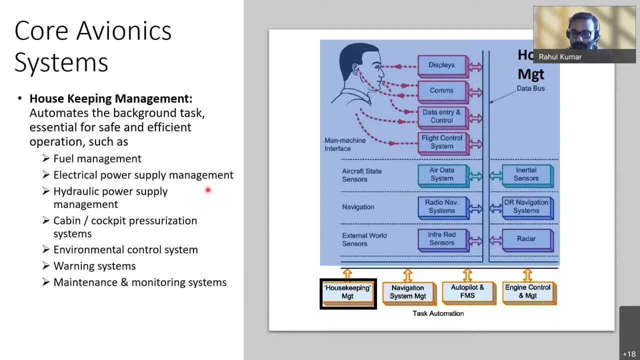 electrical power management system, then hydraulic power systems and keep in pressure. and then, when that is done, we have the cockpit pressure system which controls the pressurization of the cockpit, and then you have environmental control system which maintains the temperature and humidity within the cockpit, or even in civil aircraft also they are used. then you 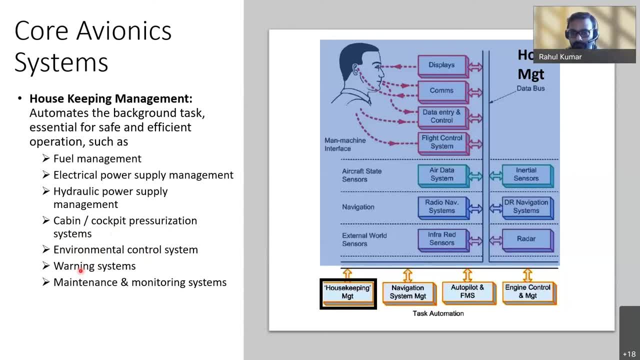 have some warning system right. so this would include both the visual warning, maybe flashing light, and the voice warning right as well, the sound as well, and the maintenance and monitoring system. so all these subsystems they are included in in this housekeeping management system which kind of monitor the overall working or the performance of the aircraft. 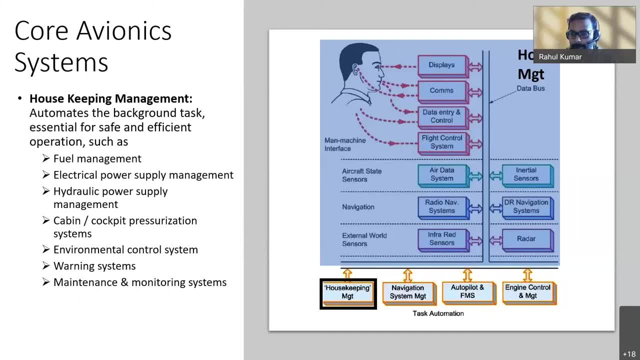 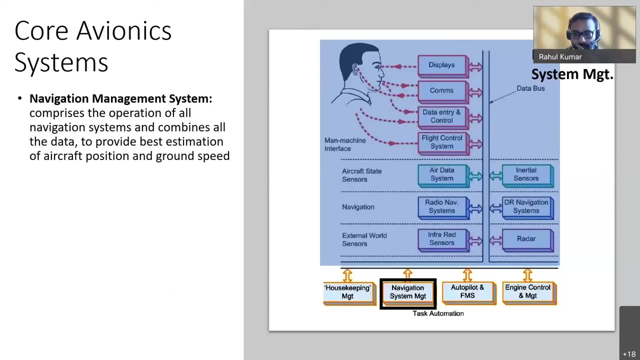 then you have navigation management system. so in the previous slide we have discussed different navigation systems, right? so the information from all those different sources, they are combined by the navigation management system and it will process. basically it will be computer. it will then monitor your navigation issues if there is company faze at the airport. 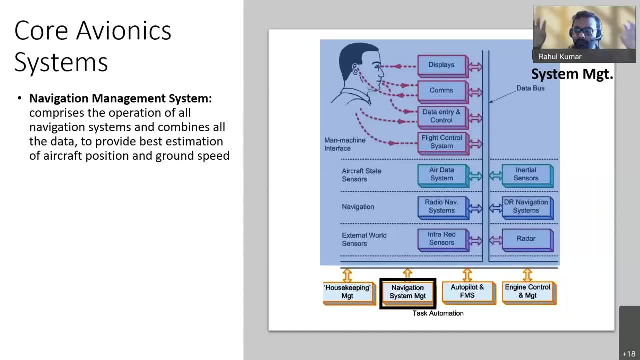 process all the navigation information from different navigation systems and it will process or combine all the data to provide best estimate of the aircraft position and ground speed. Okay, so, from different sources it will collect the navigation, process it and provide the best estimate of the aircraft position. 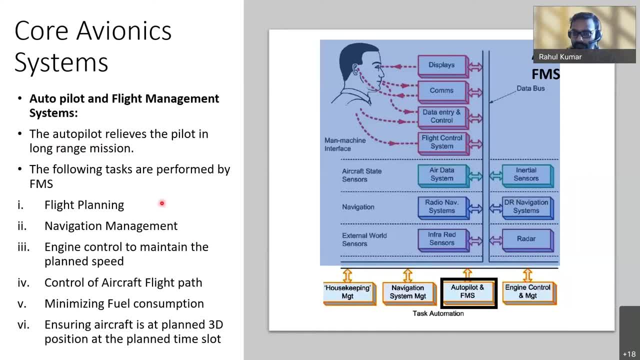 Then you have autopilot system, which is quite common in most of the commercial aircraft. So this autopilot system, basically they can be operated in various modes. You would have height hold. You can operate the autopilot system In height hold mode. 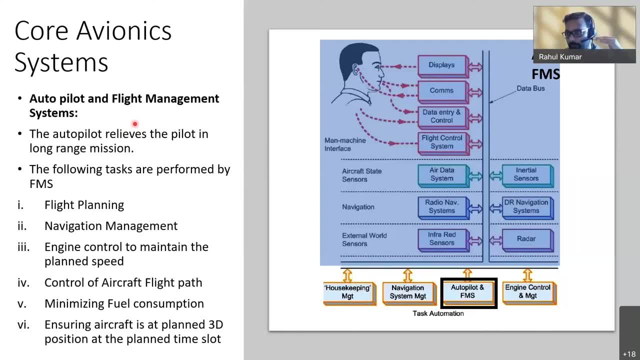 So it will maintain the altitude of the aircraft right. Then you can also operate in heading hold, So it will. if it is flying at a particular heading, it will continue to fly in that heading right. So basically, autopilot. they can be operated in these two modes and also they can assist. 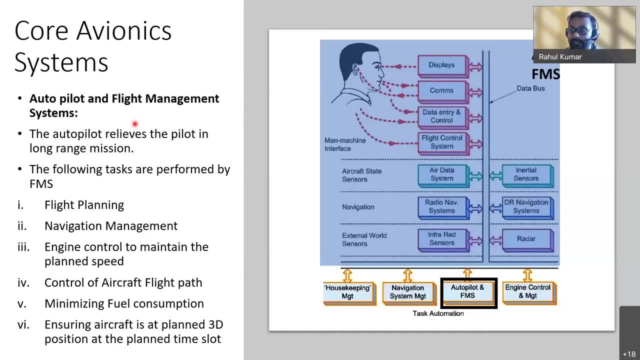 the aircraft. They can also assist the aircraft in automatic landing, So while the aircraft is landing, it can. that can be also done automatically with the help of this autopilot avionics system. Okay, And then along with that, you have flight management system, or, in short, we call them. 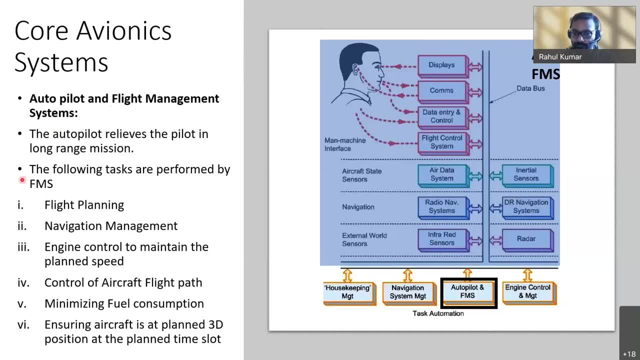 as FMS right Flight management system And basically they The flight management system. it reduces the work of the pilot significantly, So it will do the flight planning. So if the pilot just enters the GPS coordinates of its destination, the FMS system will give. 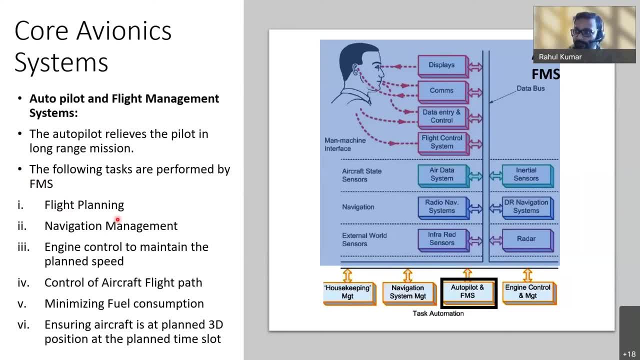 the best path which the flight can follow, and it will also give information on the fuel the aircraft should carry to reach its destination. Okay, So all those information will be calculated or it will be given by this FMS system. It will also provide navigation information. again, it will also provide, or it will control. 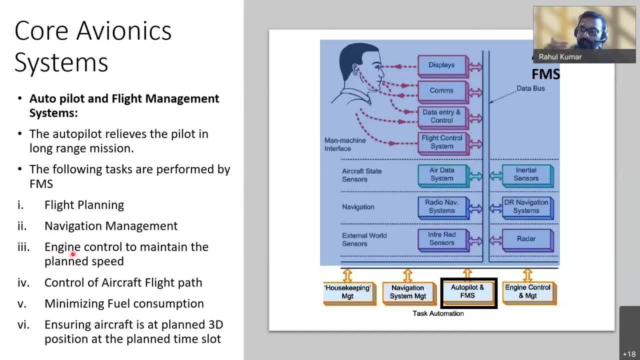 or maintain the engine. So during the flight it will control the flow of the fuel or it will minimize the flow of the fuel. It will also minimize the fuel consumption. So basically, when the flight takes off it is heavy because the tanks they are full. 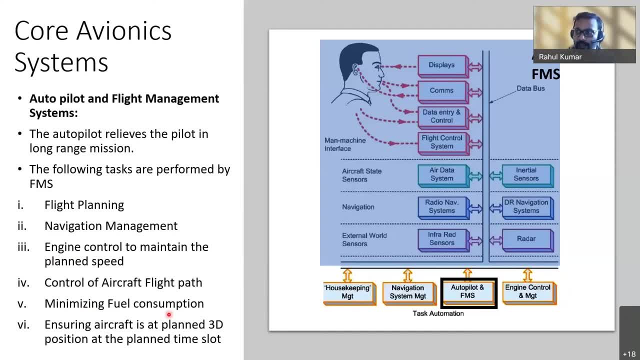 You have fuel. it is carrying the most amount of weight, But as it approaches the destination, or as it flies towards the destination, it will burn the fuel right. And when it approaches the destination the aircraft is lighter. So if the aircraft is light in weight, so it would need less amount of fuel while landing. 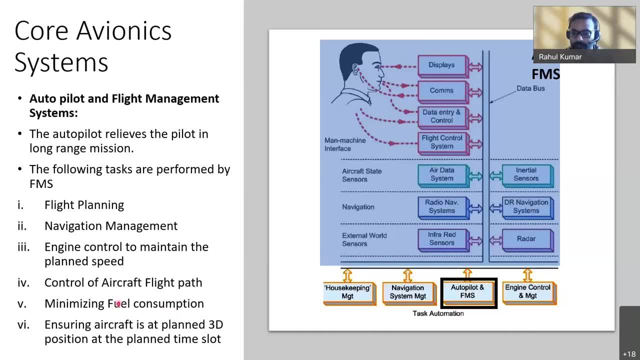 right. so that is controlled by your fms system. so it will keep on tracking the weight of the aircraft and it will accordingly adjust the fuel consumption, right. so obviously that will make the flight or the aircraft more efficient and it ensures the fms system. it will ensure that the aircraft is at the scheduled 3d position, right. 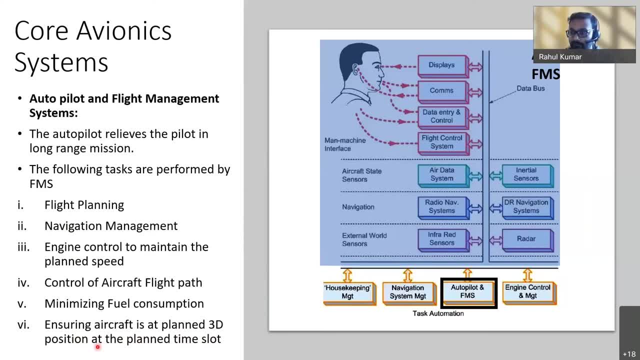 so it will ensure that the aircraft is at planned 3d position at the planned time slot. so for air traffic control, or nowadays, with you know, with the increase in air, air traffic, these- it is quite necessary to know the exact location and plan the flight right. so it is essential for the air. 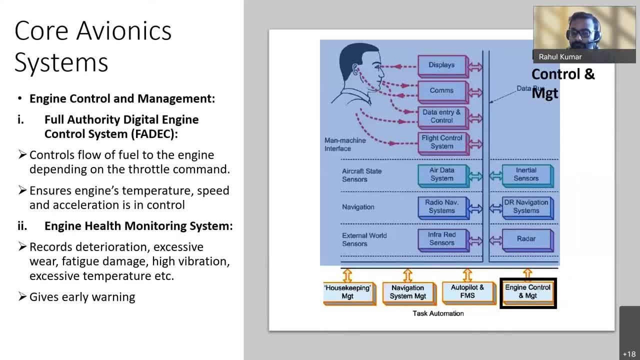 traffic control system as well. uh, the last avionics system is your full authority, the digital engine control system so, which controls the flow of fuel to the engine. it ensures that the engine temperature, the speed and acceleration is in control, right. it monitors the engine and it also is used for engine health monitoring, right? so? 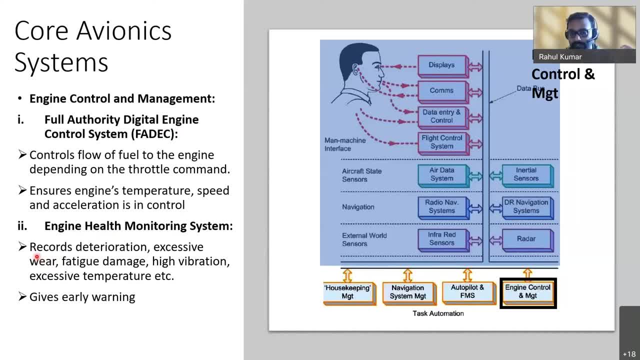 it will record the deterioration or any excess wear and tear in the engine and inform the the pilot if there is a warning, or it will also inform the maintenance engineer as well. right, so it keeps the track of the engine and it will provide, it will monitor the health of the engine and it will 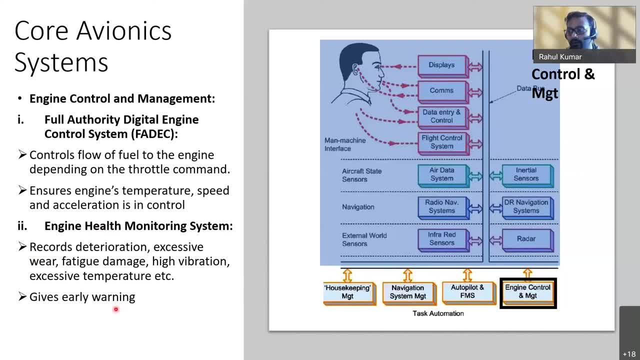 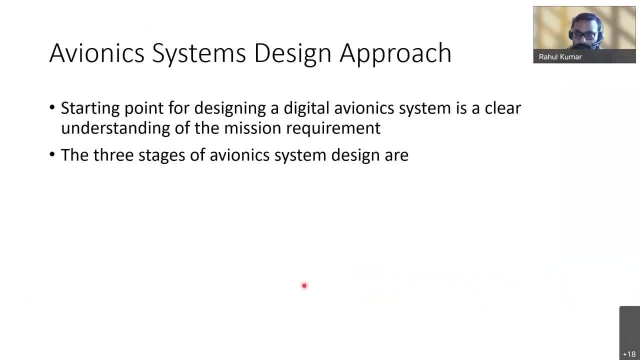 provide the warning to the pilot or to the maintenance engineer? now to design an avionics system, the first thing is, or the starting point is, a clear understanding of the mission requirement, right? what is the purpose of the mission? right? what is the purpose of designing that avionic system? 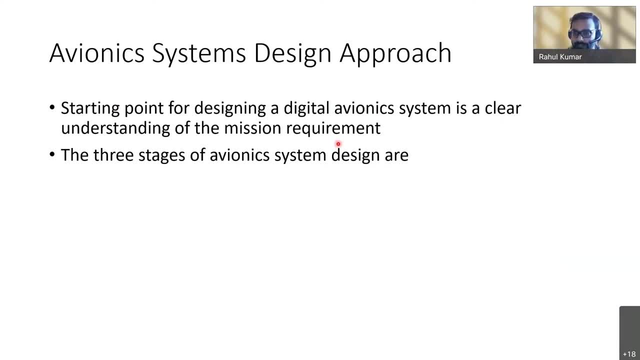 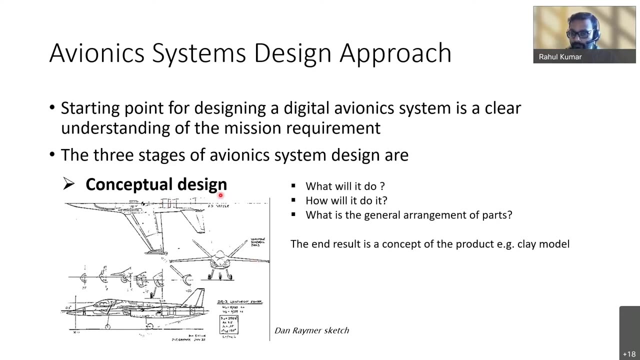 right. so once that understanding is there, then there are three stages in which avionic systems they are designed. the first stage is your conceptual design, so in which the design engineer, it will answer some of these questions, that what that avionic system will do, how it will do and what is the general arrangement of the part. 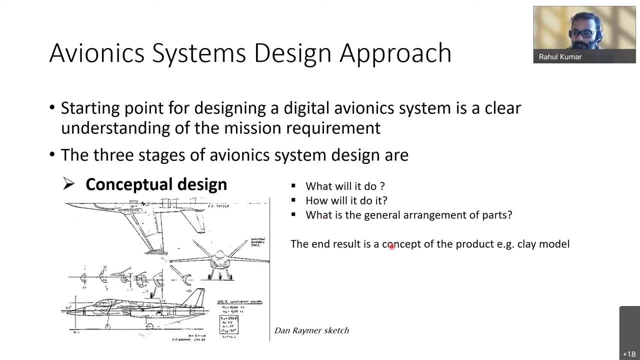 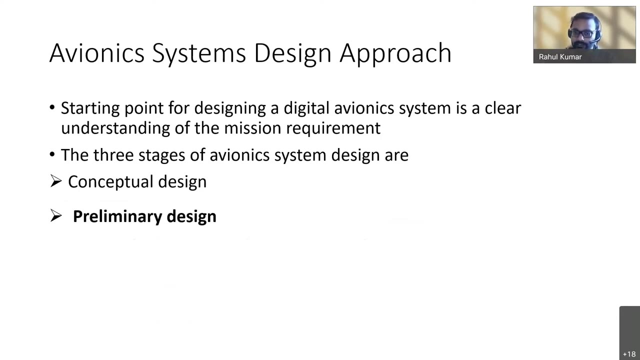 So generally the end result is a clay model or a sketch, something like this. After the first step, you should have that conceptual design in form of a sketch or a model. The next stage of designing an avionic system is your preliminary design. 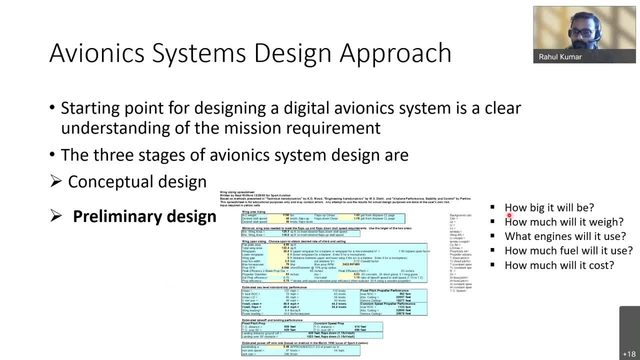 So in this stage you have to consider that- how big it is going to be- or you have to consider all the details of the individual part, like how big it is going to be, what will be the weight, How much it is going to cost, right? 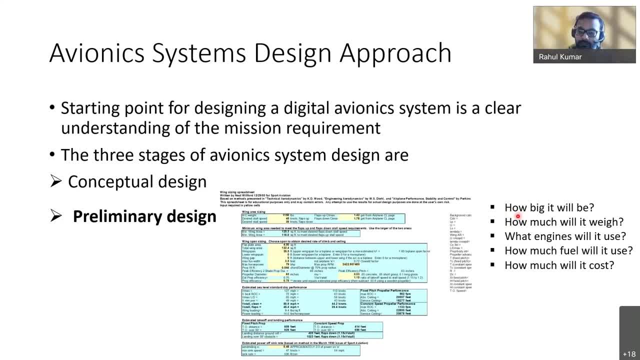 So all that analysis is done. So generally the end result is a spreadsheet. So generally this preliminary design analysis is done on a spreadsheet, So you will kind of estimate the weight, the size of the avionic system and how much fuel it may consume or what will be the cost. 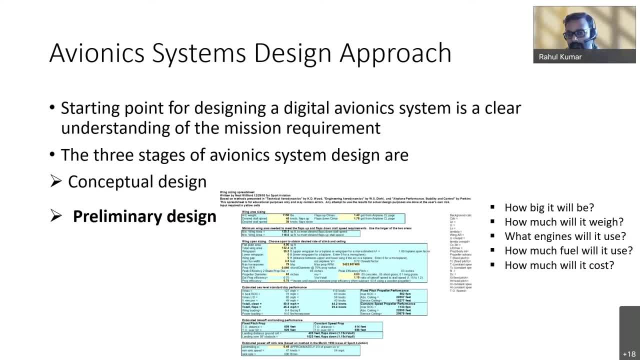 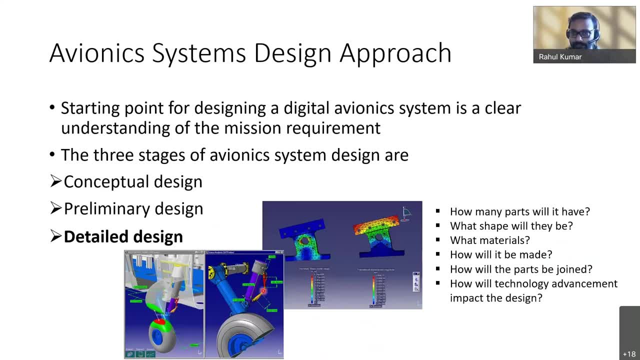 After you have done this analysis, the next step or the next stage before fabricating the avionic system is your detailed design stage. So in this generally, we develop a model or a simulation model right, And in the software, we develop a model or a simulation model right. 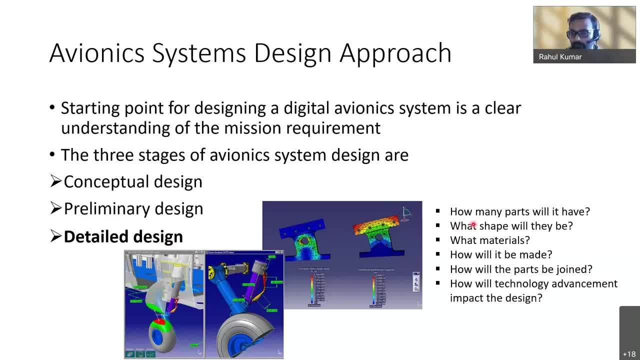 So we test that model, whether you know how many parts it will have. what are the material which we could use to fabricate that avionic system? So something like if you are designing an avionic system or any part for a military aircraft right which flies at very high speed. 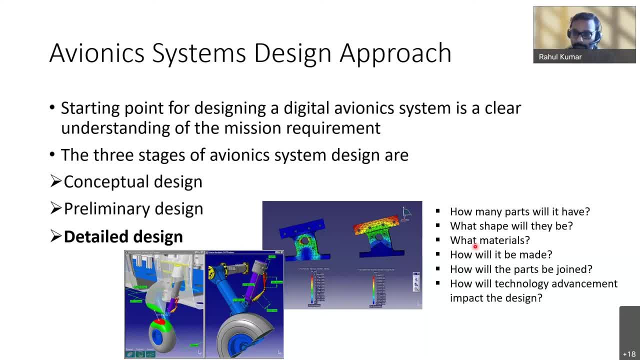 They are designed to fly at max speed or the speed of sound, right. So if you are designing any equipment for military aircraft, you should consider that the aircraft would or could fly at very high speed. So whether the material which you are using will it be able to withstand that amount of pressure or drag. 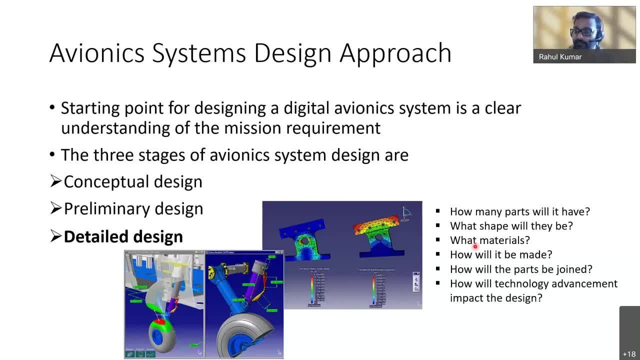 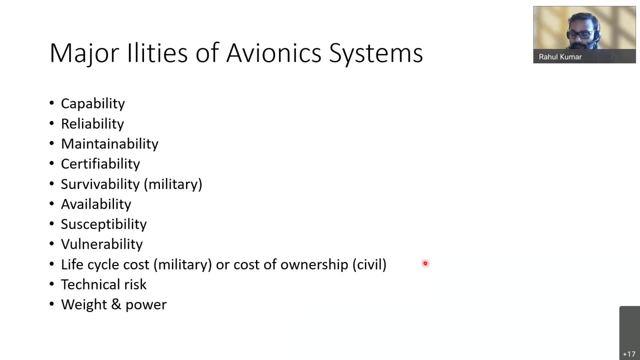 When the aircraft is, When the aircraft is flying at that high speed, right? So you have to consider all those factors in the detailed design part. Now, finally, along with those design steps which I have mentioned, basically three steps- 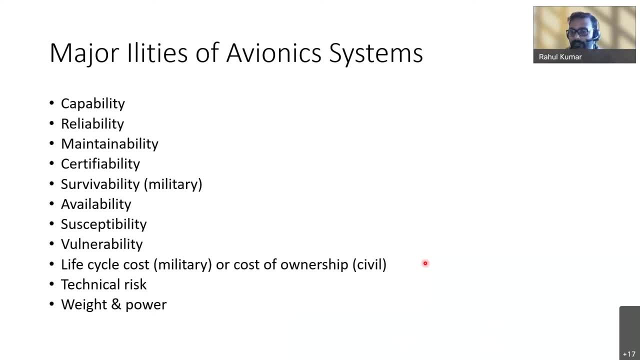 we also need. We need to consider some of the elites which the avionic system should have. So elite, basically it means the quality the avionic system should exhibit or it should present, right. So these are the qualities, some of the qualities which an avionic system should have, right. 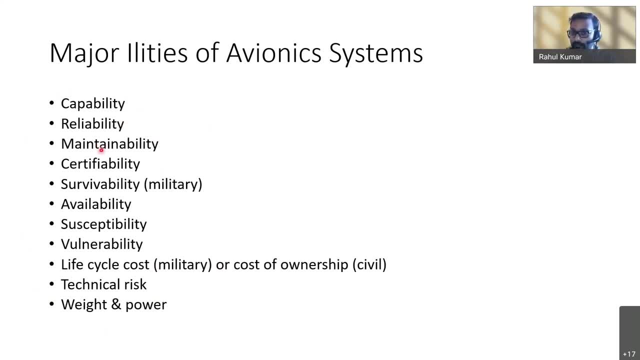 It should be obviously reliable, It should be maintainable, That is, if you know that avionic system stops working, you should be able to maintain it or repair it. Then there is certification. So generally all the aviation or avionic systems, they are certified by some authorities, right? 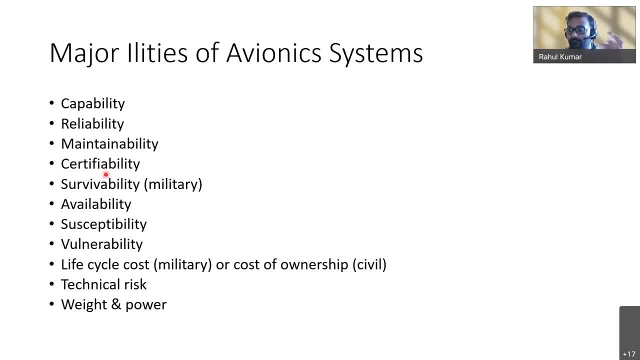 So if, while designing the avionic system, we should also We should consider that whether it is going to pass the certification or not, then in the case of military aircraft, you should also The avionic system should also be considering survivability, that in the adverse condition, or in very high speed or in such adverse condition, whether my avionic system is going to survive or not. 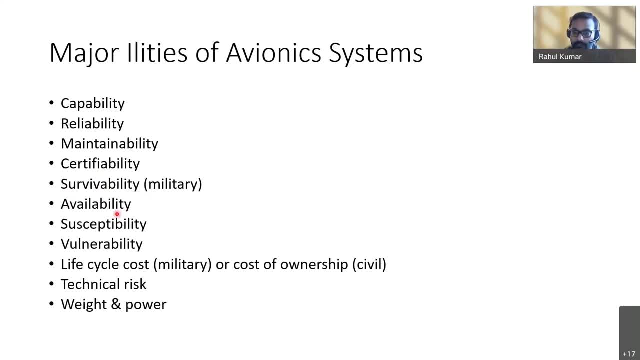 Okay, Availability obviously is quite important. So if you have to replace the avionic system, it should be easily available. Then you have life cycle cost in military or cost of ownership. So while designing an avionic system you should also consider that maybe you have that concept of designing a very high end avionic system. 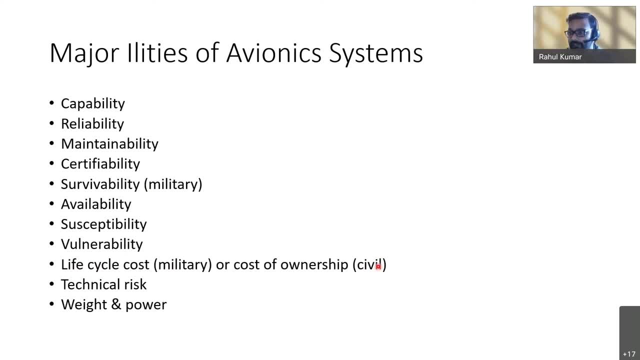 avionics system, very sophisticated avionics system, But you should also consider the cost of ownership. If that avionics system requires continuous maintenance or if it requires replacement after a very short period, then it is going to cost a lot for the company. 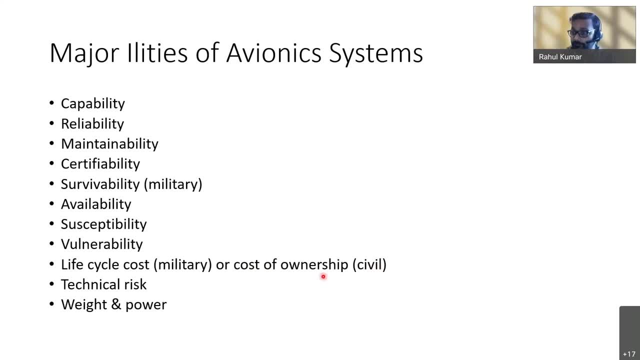 Right, so that is your cost of ownership. So we should also consider this while designing. And obviously, technical risk: no sparking, no fire, right? all those or it should provide the accurate information, So such type of technical risk should not be there.